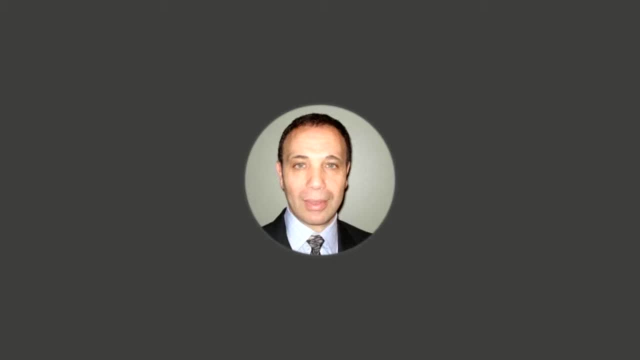 All right, Please have a look at this one. The question is: what is the ultimate goal of a company? Here is the poll. Please go ahead and think about that for a few moments and then chime in with your vote. I see I spelled the first one incorrectly. That should say develop new technology. 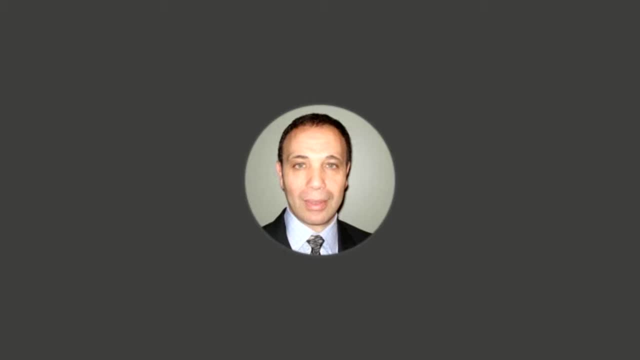 The vote is already done. We're not able to select any. Oh, that's, that's unusual. OK, well, let me let me kill this one and I will redo it See if. Yeah, I don't like getting anything either, So let me try that again. 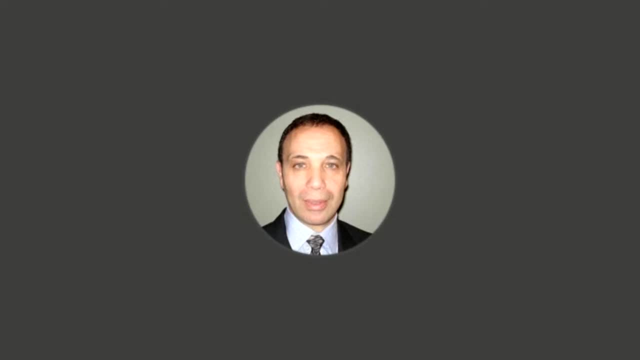 I'm not sure what went. What happened with that one? OK, here we go. I have a clear, a clear one, So let me try it again So you can start thinking about it. you have an idea of what I'm going to be asking. 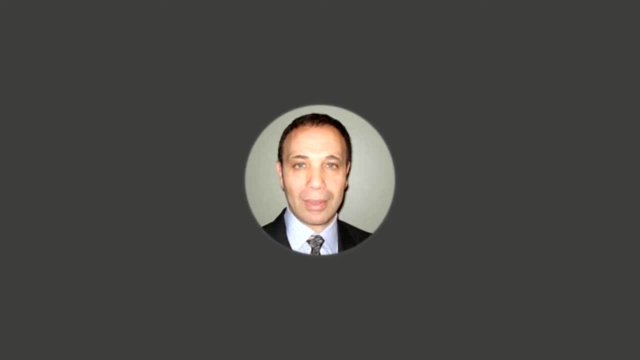 OK, here we go. And one more, Here we go. Give that a go. That should be working now. OK, I see you're all chiming in. I'll give you a few more moments. OK, fantastic, I see that many of you have given me your choice for the answer. 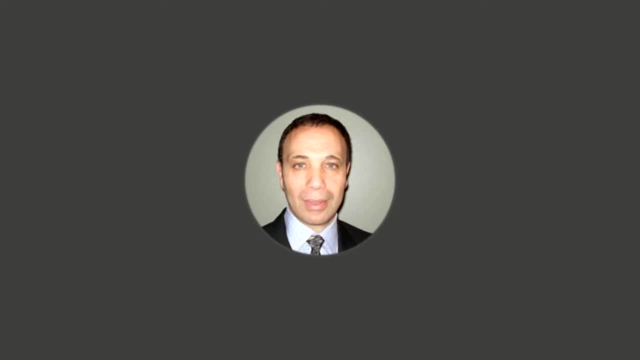 So let me show you the choices you've selected. So we have three people who did not respond. We have one person who chose develop technology for people who selected make money, No people selected make products And ten people- the majority of the people respondents- said all of the above. 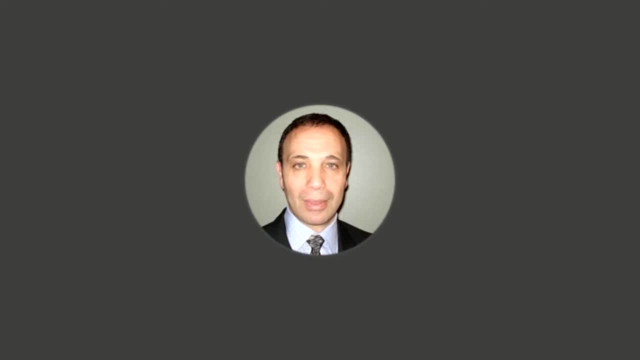 So That is a- this is rather interesting question because it's rather open ended and it's a little, I would have to say, misleading. So Let me qualify this a little bit, And I do appreciate that many of you said all of the above, because 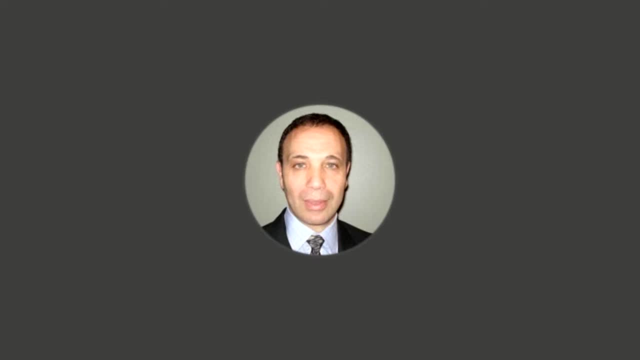 Definitely The role of a company. once a company is in existence, they have to develop technology to keep existing, continue existing and to move forward. They have to. they have to make products because that's how they make their revenue And obviously they also have to make money. 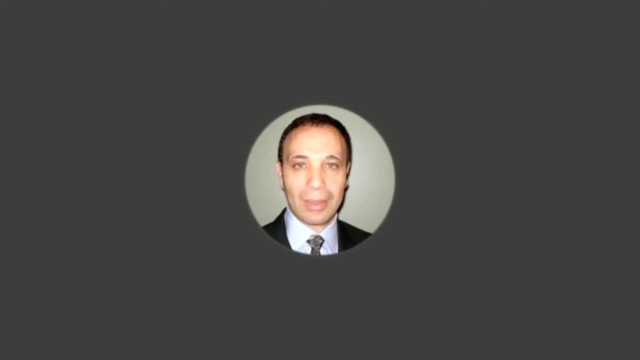 So it's easy to say all of the above, But I want to clarify this point a little bit further and just look a little bit deeper. If I were to ask you what is the ultimate goal of a company, The answer, I think, is a little clearer. 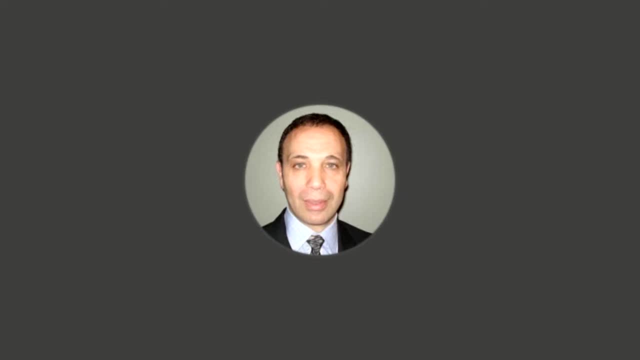 The ultimate goal is to make money. Simple as that. Of course, as I said earlier, companies have to develop new technology to remain competitive and remain leaders in their field And of course they have to make products. But you know, I put there as many as possible. 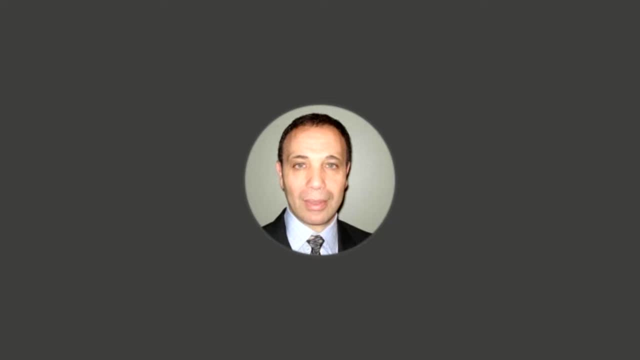 And that may not necessarily be a true statement. We will see this later in the course. Why that may not be the case, But yes, we do want to make products. So The all of the above response needs a little bit of clarification. 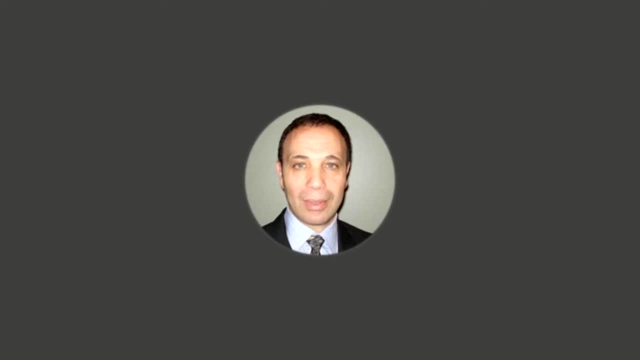 So I would say to you: the ultimate goal of any company is to make money. how we make the money, that may be addressed in different ways, All right. So that was a little bit- Let's call it- tricky. Thank you for doing that. 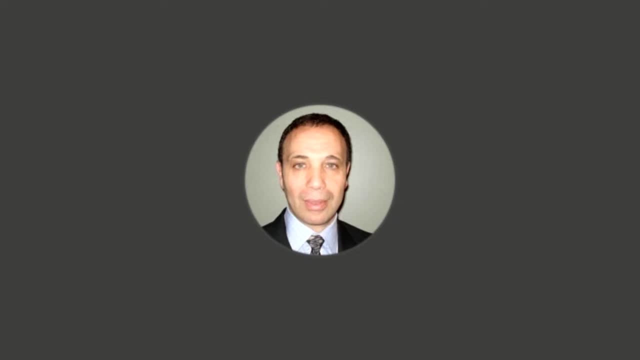 And I want to ask you one more, and then we'll move on to the actual presentation. So let's do another quick poll, Also multiple choice here, And this one. the question I am going to ask of you is the following: We're going to 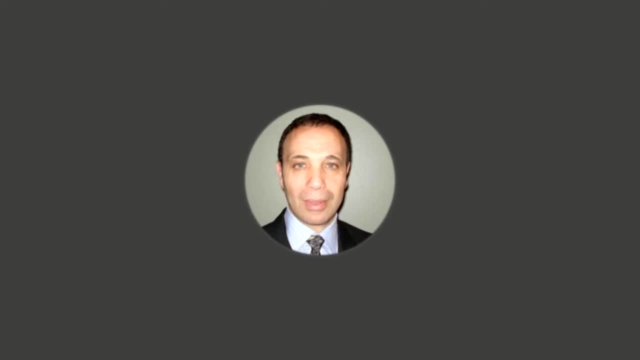 What must companies do To stay in business? So you can start thinking about the question. I'm going to put down the answers that I'm going to suggest for you And I'm going to put down four options for you. And I'm almost getting there. 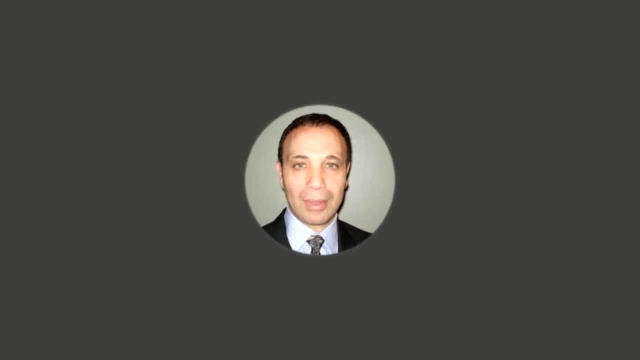 So just bear with me, All right. The survey, the poll, is complete. I'm going to share it with you And go ahead and please submit your responses, All right? Okay, A few more moments. And Okay, A few more moments. 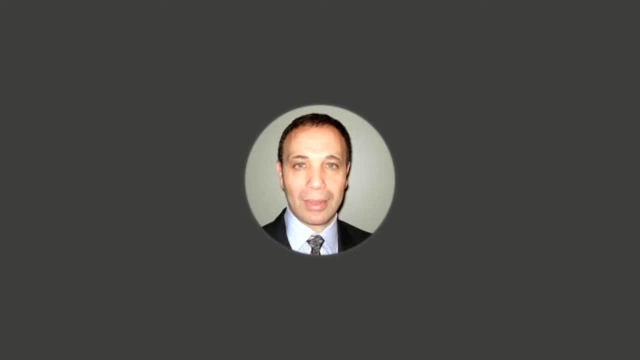 Kyle chums in. It's tricky. All right, Let me. It looks like the majority of you have given me a response, So I'll share it with you. Share the results. Here we go. I have two no respondents. Four of you said: make high quality products. 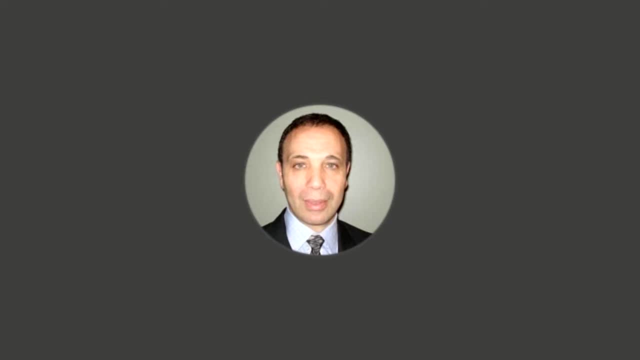 Nobody selected number two, which is market new products fast, And no one selected number three, which is reduce Costs, And the majority of you, 12.- Selected All of the above. Congratulations to the 12 who selected all of the above. 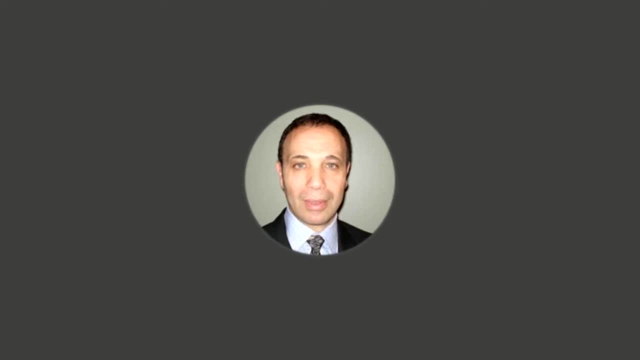 So, if you think about it for a moment, Yes, We must make high quality product products If we want to maintain our customers. Two, We have to market new products and we have to do it Fast. We have to, We have to. 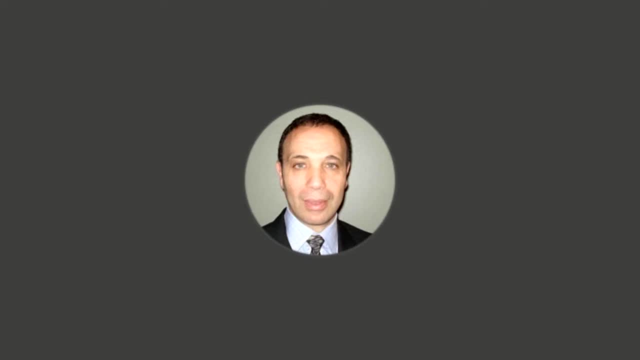 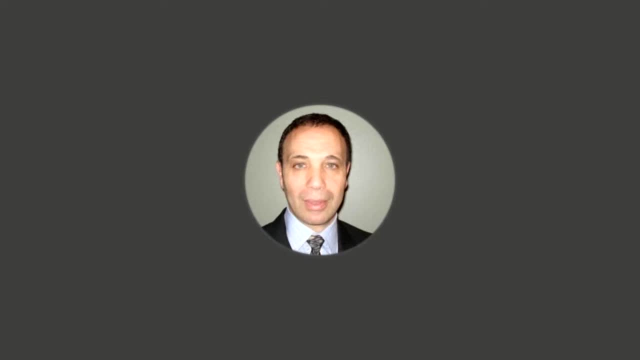 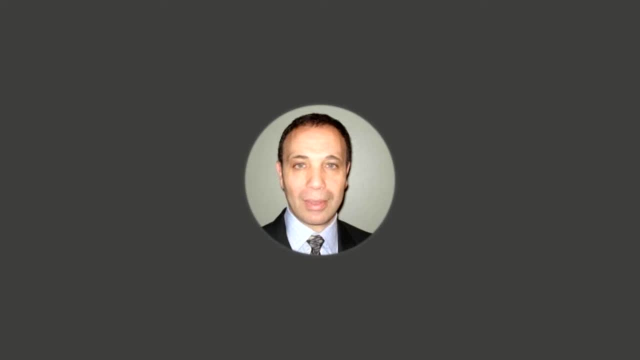 So the correct choice for this one would be all of the above, and we're going to talk about all of these in a moment. So this is a good segue into my lecture for the second half of our session today. So let me close the poll. 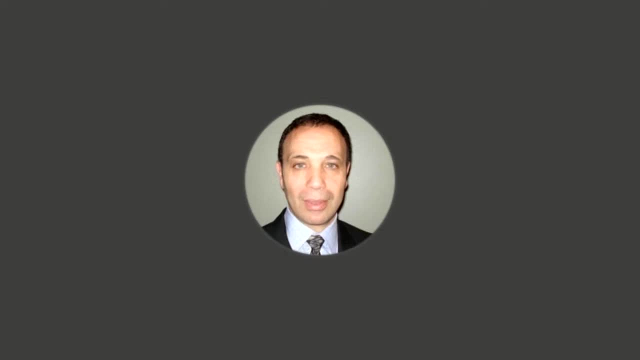 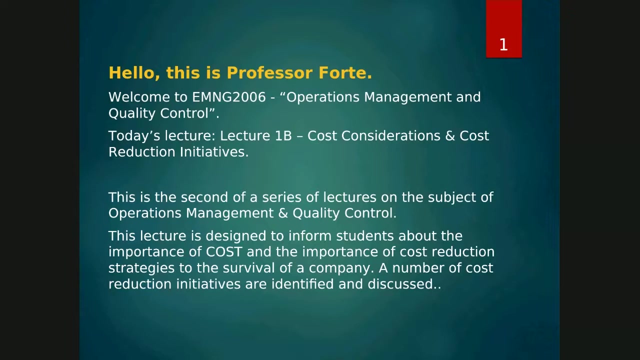 and I'm going to open up my second lecture and I'm going to share it with you now and here it comes up one moment, all right. so today's lecture, this is lecture 1b. the title is cost considerations and cost reduction initiatives. as noted here, this is the second of a series of lectures on the 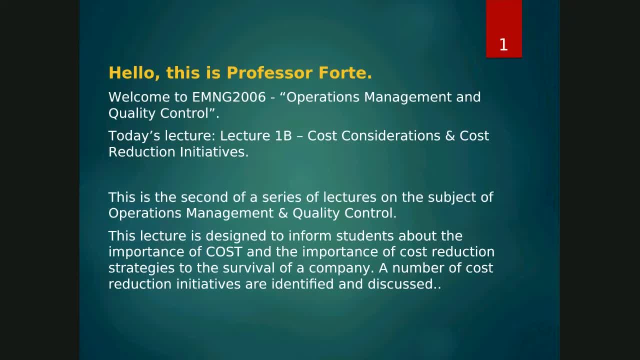 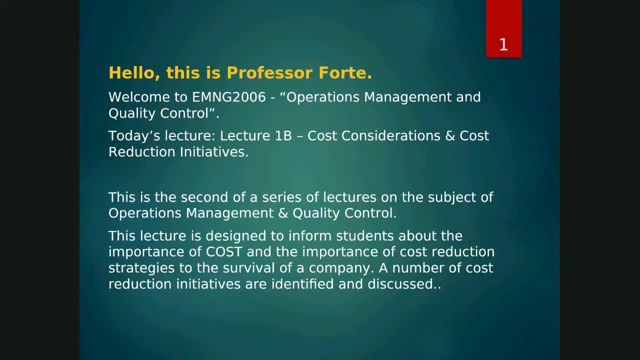 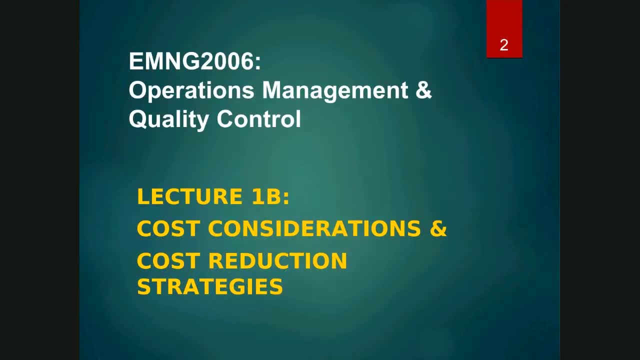 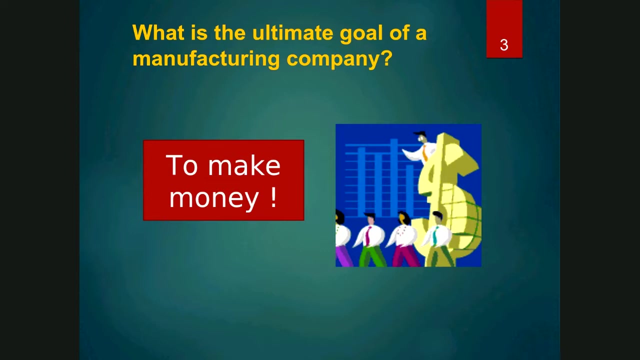 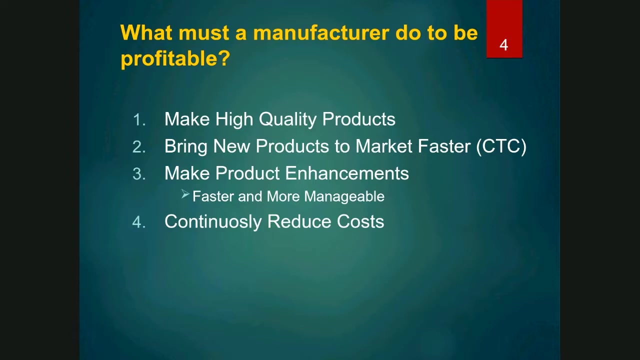 number of cost reduction initiatives are identified and discussed. alright, so here we have it, lecture 1b: cost considerations and cost reduction strategies. so the ultimate goal of a company to make money. so this was a second poll question: what must, what must manufacturers or companies do to be? 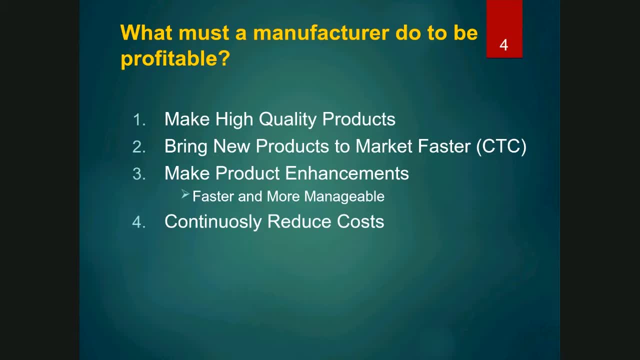 profitable. so here's the list for us. we had these on the pole so we could. first of all, we got to make high quality products. if you think, when you go out and buy a brand or something, if you don't think that it's a good quality product, you're not going to spend your money on it, not at least for. 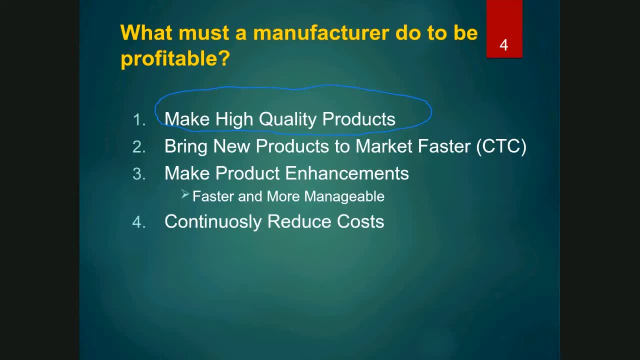 products that are important to us. we have to be able to introduce new products into the market and we have to do that fast. the example I like to use here is: think about it, Apple, and I'm sure that in the last five years, if you just think about the last five years, how? 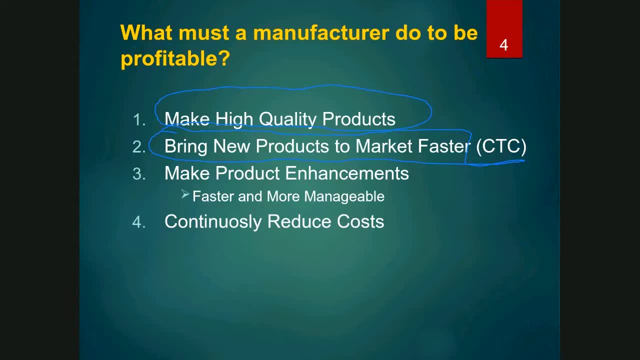 many iterations of the iPhone have there been? does anybody know what level they're at? but all I think is, yeah, there's a new iPhone every year, or even even faster. absolutely. you and I think Kyle suggesting iPhone 11 is the latest and the greatest. I'm not even sure I've 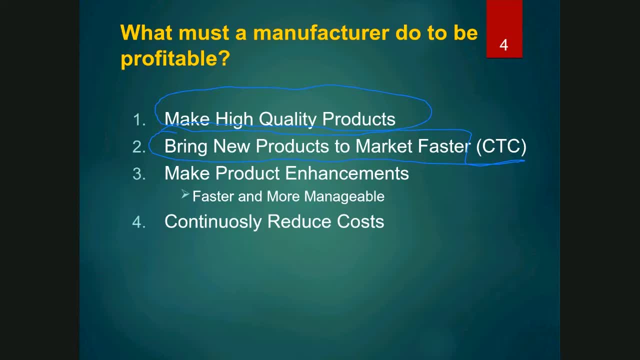 lost track, but I know that every time I go to replace my phone I I see there's a new generation of phones, not only from Apple, but all the other manufacturers- Samsung, LG, you name it. they all have new versions really quickly. this is an important consideration. um, there is something. 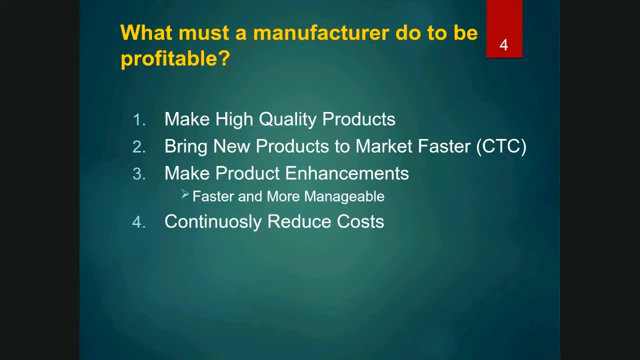 that we used in automotive, and I'm going to talk about this later. this acronym here, C2C, is actually- I'm going to write it up here so you remember it. it means concept, concept to whoops. pardon me, I'm trying to type with my mouse here and it doesn't really work that well. 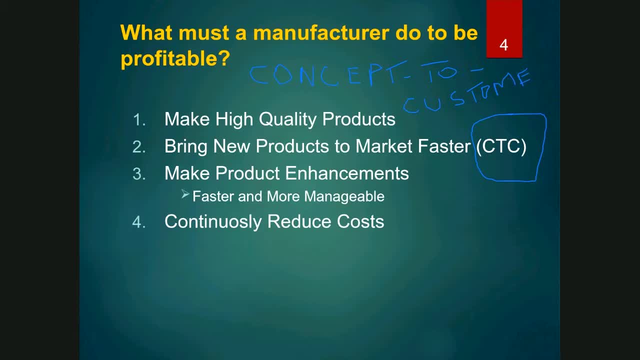 that's the acronym right there. CTC stands for concept to customer. what we mean by that is the time frame that is involved, from the time, the initial time that we have a concept for a product, an idea for a product, to the time that we actually are able to design, build. 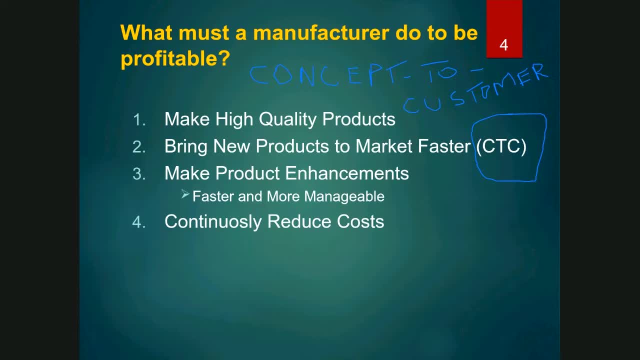 put out to the market, to our customer. so that entire time frame from initial idea conception to the time we get the product out to the customer is called c t c: concept to customer. the idea here is that if we can make that time shorter and shorter, then we're able to get new product, new product. 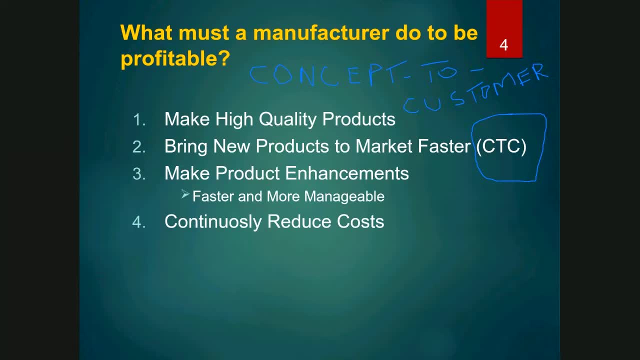 ideas to the market faster and faster. so the question, obvious question to you is: why do you think apple wants to put a new iphone out there every year? and the obvious question is because people want to buy the new version, and every time they buy a new phone, obviously apple makes more revenue. 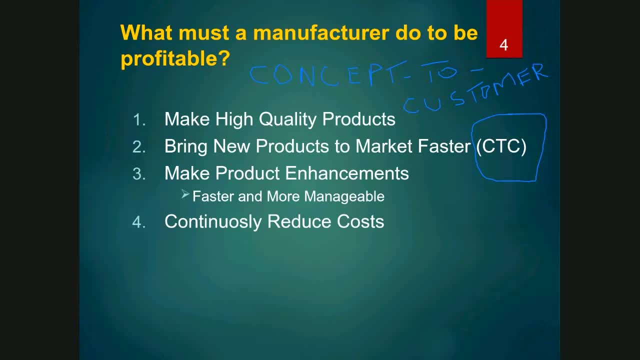 and not only true of apple, but that is true of everyone. kyle chimes in and says: you want to keep your customers interested. very true, good point, kyle, but the bottom line is they make getting more revenue from this. so when i was in the automotive 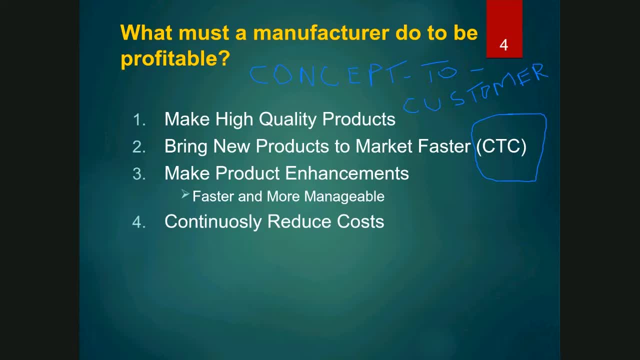 industry. i was in the mechanism designing elec we. the c t c time frame they used was four years. so they they came up with an idea of what they wanted to do to create a new model and by the time they got it to to the customers, it was a time here, a four-year time frame. they realized that four years was hard after long time with, but in fact it wasn't. lastly, they saw that it was more than four is a long time before they learned. later, and beyond this car and the much longer they knew that for the rest of ten days they work were happening all by different companies and- and that's concerning how we were able to keep up with what they needed, and they've caught many. three, seven years of price, ten years, not what we saw. we haven't done anything. they doing. i couldn't be in clone. they even suggest one of seven days because, because you wouldn't do it. so, yeah, ten years of two years. we were 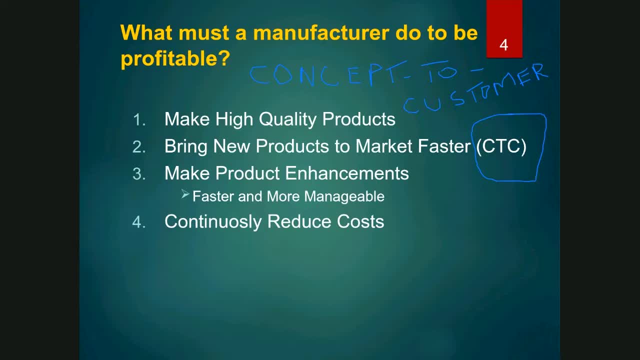 They realized that four years was a long time and the models got a little stale. after four years People get like Kyle said: you lose interest. So they realized that four years was too long. So they changed that. They tried a new target that said let's try to get a new model out there every three years. 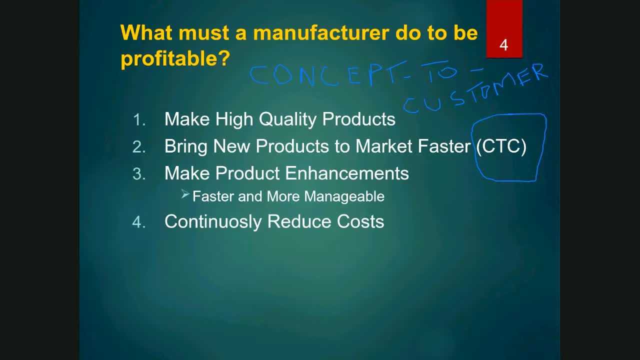 And then, after they implemented three-year CTC, they said: well, let's push for two years, And by the time I left Ford, we were working on a two-year cycle. Try to come up with new ideas for new model cars and get them out there in two years so we can turn around our car vehicles, our vehicle models, much quicker and keep the interest of the customer and keep selling new models more and more. 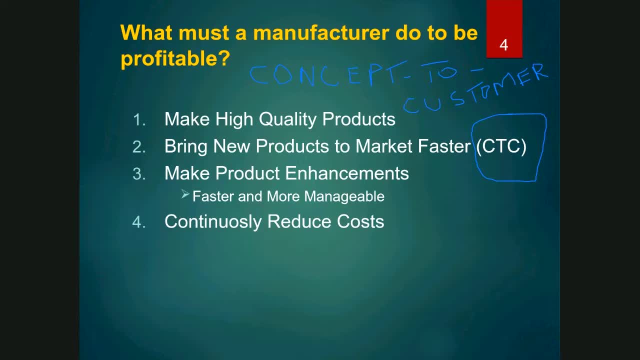 That's where the money comes in. So we're going to revisit this a little bit later, but I just wanted to kind of elaborate a little bit on the CTC idea. So the next point- what must manufacturers do to be profitable, or companies do to be profitable- is, along with item point number two: we also have to be able to create product enhancements. 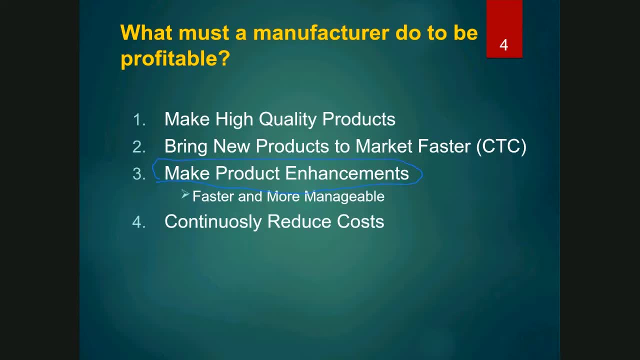 Product changes faster, more quicker and make it very manageable, very easy process for us to do And lastly, very important, we have to continuously strive to reduce our costs. Very important. So these four things, or four actions, are very important. 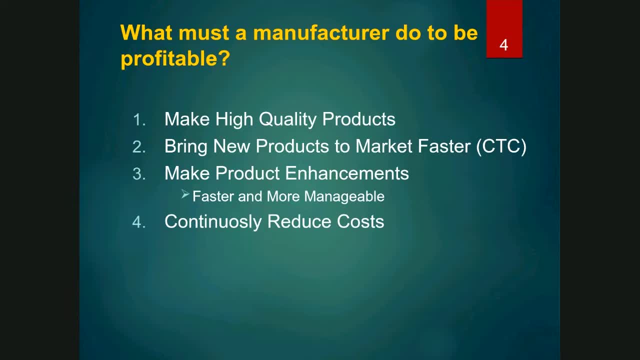 To ensure the survival or success of any company? Hi, I had. When you say reduce cost, production costs- or is it maintaining a like a product, a high quality product at a fairly reasonable cost for the customer? Yeah, Thank you for your question, Kyle. 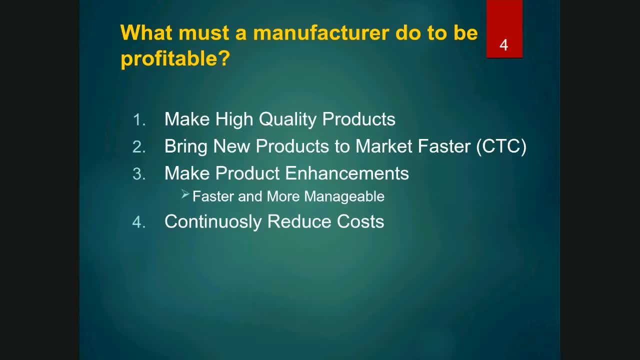 Let's let's look at the possible answers. The answers are many, so I'm not going to keep it to one short answer, but that your question is a good segue to my next couple of slides, So I'm going to ask you to be patient and we'll try to answer that question with the slides that are coming up. 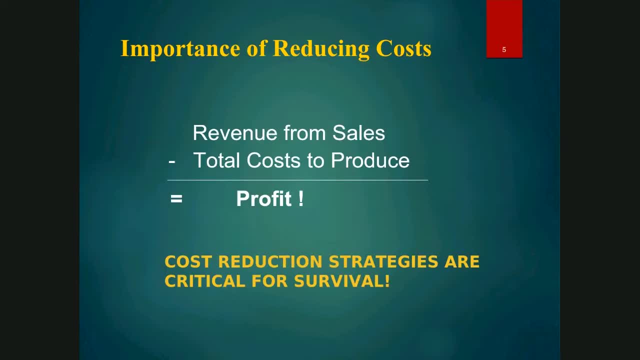 So let me the next slide. So why is it important to reduce costs? Well, the answer is very simple. We have a very simple equation here. How do we make a profit? Well, if we take all the revenues we can generate from selling our product and from that we subtract all the costs that are associated to make the product. 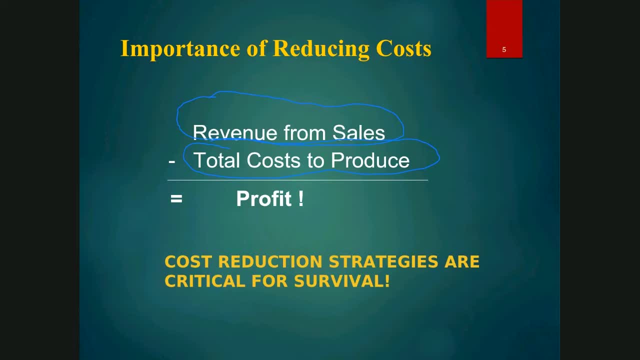 Well, what is left over is our profit. So if we're able to drive down our costs whatever way we can, then we're increasing our profits. If we increase our sales because people like our product, because we have quality products, then we increase our profit. 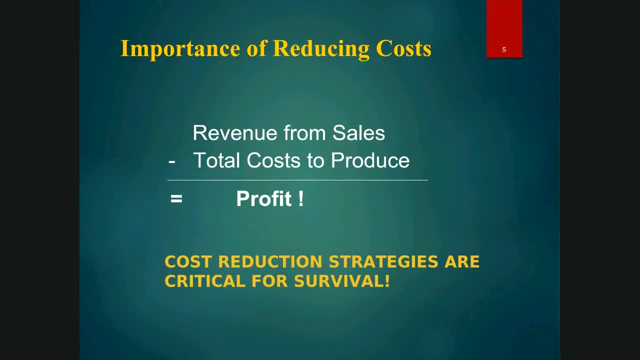 But really the point I'm making on This slide is that our challenge has to be always an ongoing challenge of reducing somehow our costs. So very important: reduce and by doing that, increase this guy, which is what we want. we increase profit. 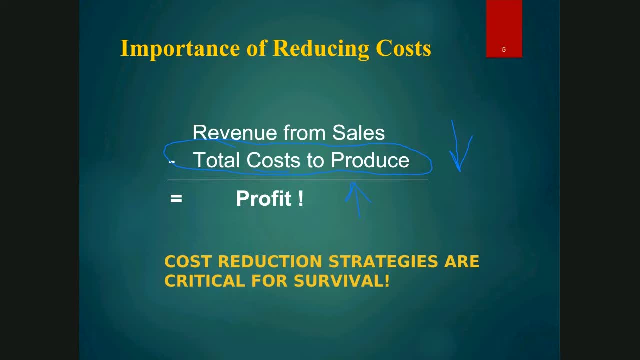 Now to address Kyle's earlier question. let's look at a couple of slides that are upcoming. So first of all, I want to Cost reduction strategies are critical for the survival of corporations, So don't let this be a mystery to you, but whenever you go work somewhere, one of the things you're always going to be asked for is: what are you doing to reduce costs for our company? 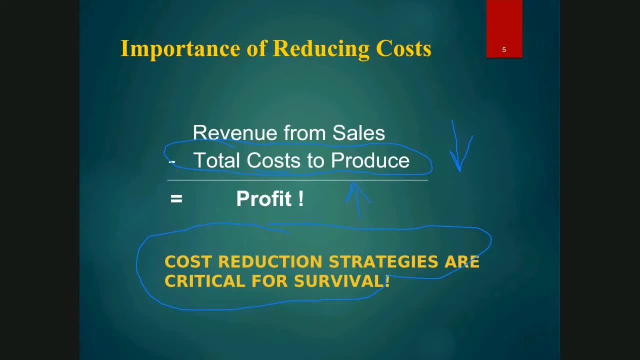 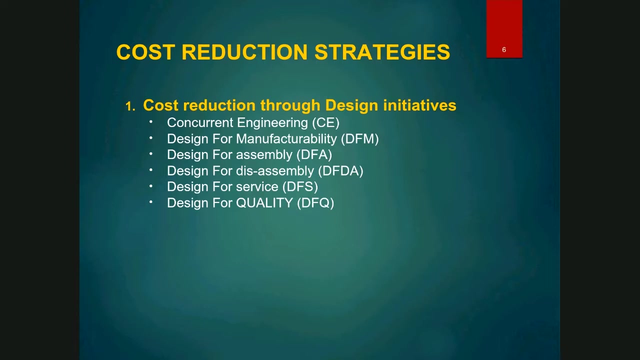 Now, you individually, but you as a group, as a team. All right, Here's our first slide That talks about cost reduction strategies. So we can move forward through these slides. What I want you to do Is think in your mind that cost reduction is not limited to one activity, and that one activity only. 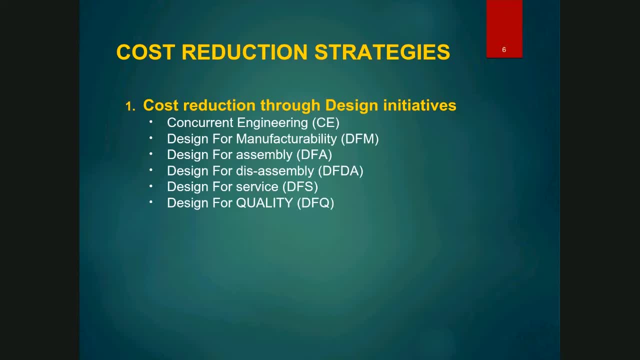 But it entails consideration of reduction strategies in all activities on our corporation. So one obvious activity is what we call or refer to as the design activity, design activity. So we have what we call design initiatives that we have to keep in mind. So let's look at the major ones. I can't talk about everything, but let's talk. 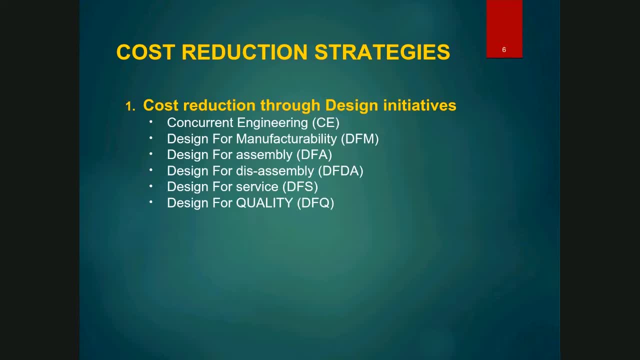 about some of the major ones. Now, some of you had me last semester as their professor for introduction to mechanical CAD and in that course I talked a lot about design strategy and how you should approach designs so you minimize costs. Now, unfortunately, I don't think I had you guys as one of my 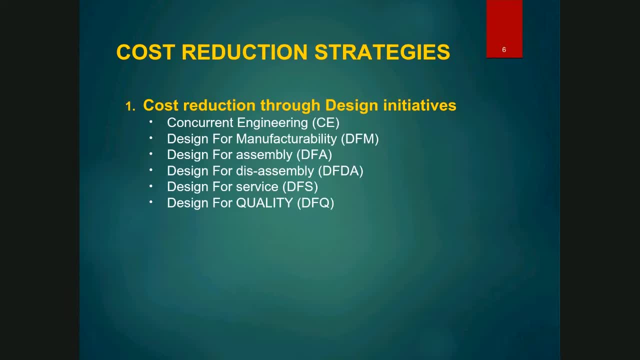 sections, but nevertheless, you did do mechanical design with someone else, so you should have an idea what I mean here. But on the big picture, when we think about design initiatives to reduce costs, these are someone that these are some of the things that we should. we should consider. First one, something 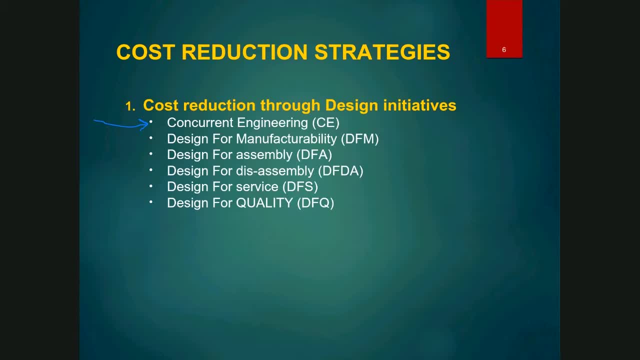 called the acronym is CE: concurrent engineering. Now, what do we mean by concurrent engineering? Again, we'll talk about this more, but for today the idea of concurrent engineering is one where you have your manufacturing activity and your design activity working together. So design activity understands what manufacturing is doing, manufacturing understands what 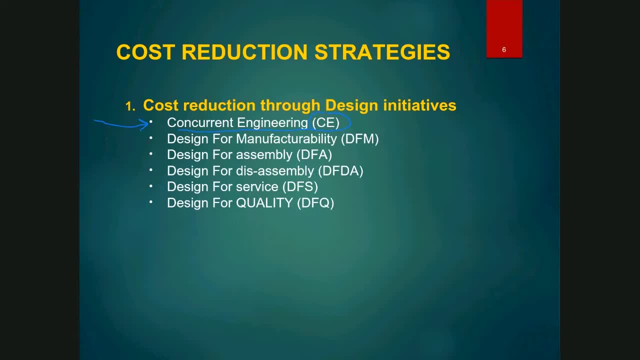 design is doing and clearly you don't want to design something that manufacturing can't do because they have a problem with your design Consulting. we can talk about what manufacturing is, but if you want to shared something- or one of the reasons is one- is the fact regarding which: 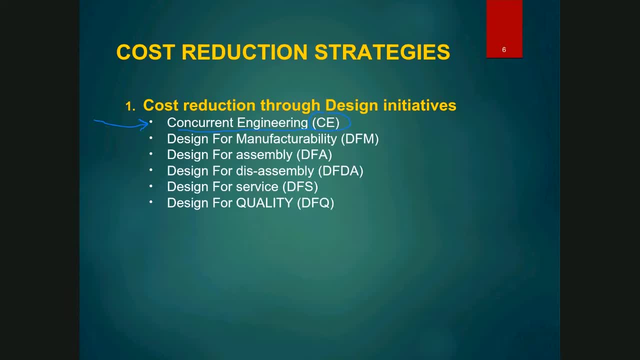 engineering means So, in which engineering means you can design in your design if you kind ofabile one or the company you're actually building, so you can design a lot of engineering by yourself if you're able, and you're able to do it. So with your design structure you can design for a lot of. 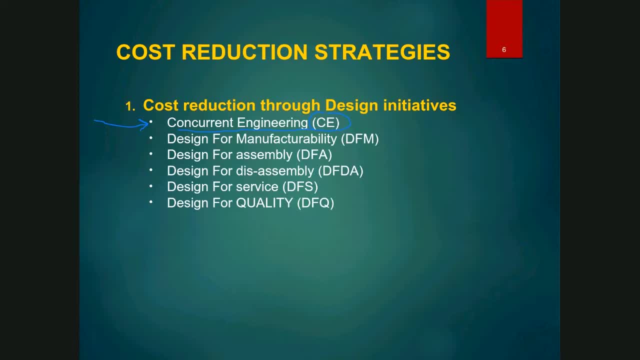 other companies in the world which can be manufactured effectively and efficiently, which leads to point number two. the idea here is called DFM, and that means design. whatever you design, you got to make sure that it's designed for manufacturability. you got to be able to make this thing efficiently. 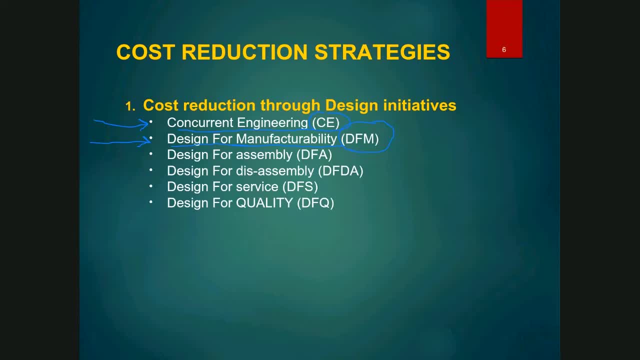 easily. so not only do we have to make something, design something that is easily manufacturable, we also have to make something that design a product that is easily for assembly. so not only can we make the parts, all the individual parts that have to go into the end product or the final product, we also 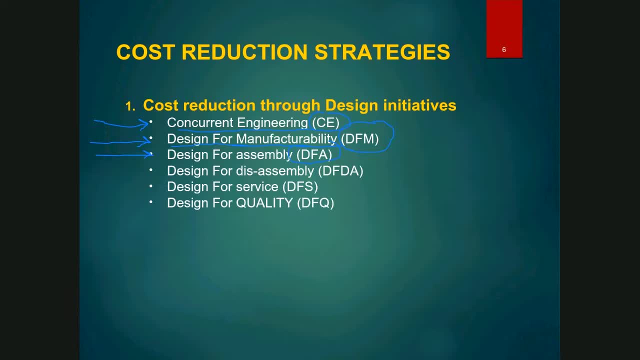 have to design the end product. so you can design the end product for the final product. you can it in such a way that it can be put together easily. so those of you who were in my mechanical design course, we saw that we designed parts and then we put. 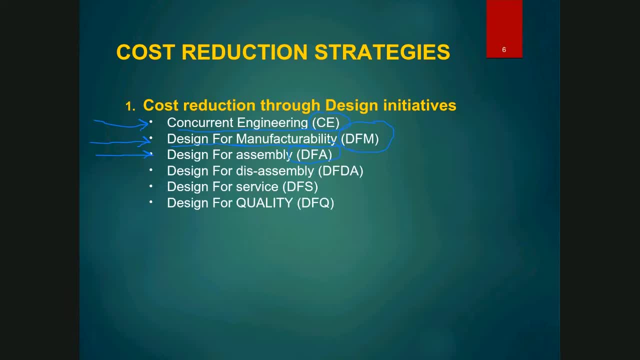 them together in assemblies, so they had to fit nicely and they had to be be able to assemble nicely, otherwise they wouldn't work. as a follow-up to that is the next consideration. when we design something, we have to design it in such a way not only that we assemble it, but we also. 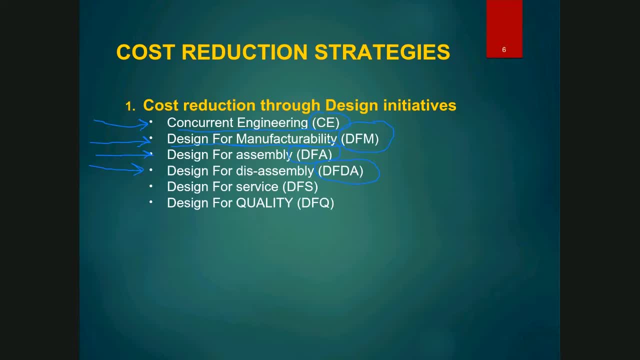 have to be able to disassemble it. so design for disassembly. so imagine you're building a vehicle, a car. there's lots and lots of parts that go into a car and at some point you figure out: oh, something is wrong, we got to take these parts again and fix that one. 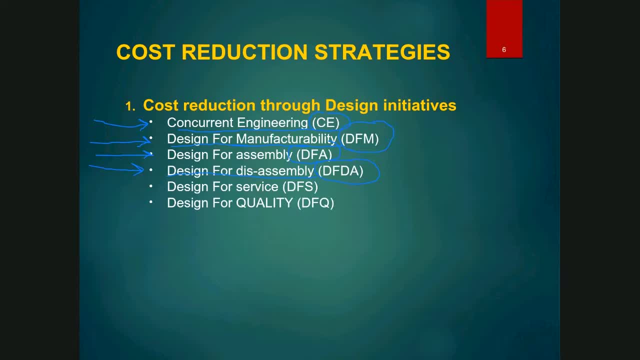 particular part. that is incorrect. if it's not easy to disassemble this, well, we're going to have a lot of problems. so we want to avoid that. we want to design it to make sure that if we can assemble it, we should be able to also disassemble. 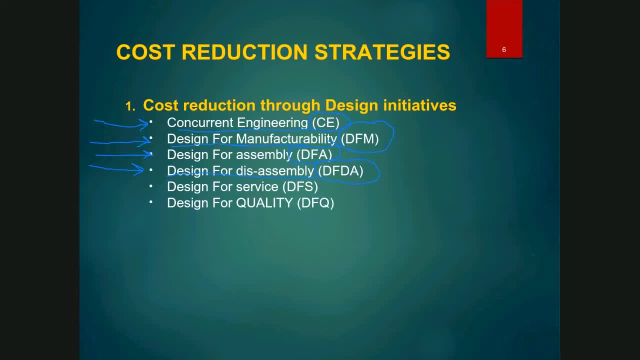 it so we can fix anything that needs to be fixed. which leads to the next point, which is more specific design, dfs, and that means design for service. so can you imagine buying a car and you can't find where you got to put your oil in? that's a bit of a problem, or how can they? 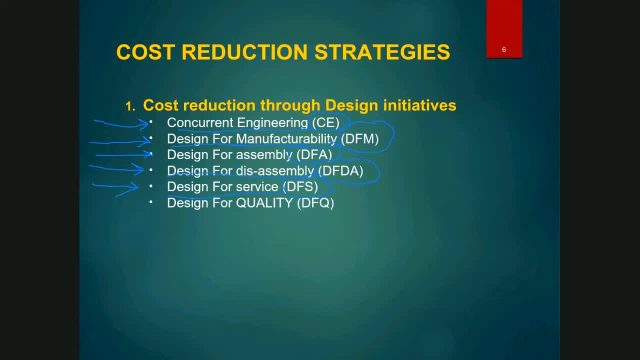 service your car. if they don't, they can't get things. i remember once i had a vehicle that was a vehicle and they had mounted the fuel gauge of the vehicle inside the gas tank of the vehicle. i'm not going to make any names here. i don't want to discredit the company. 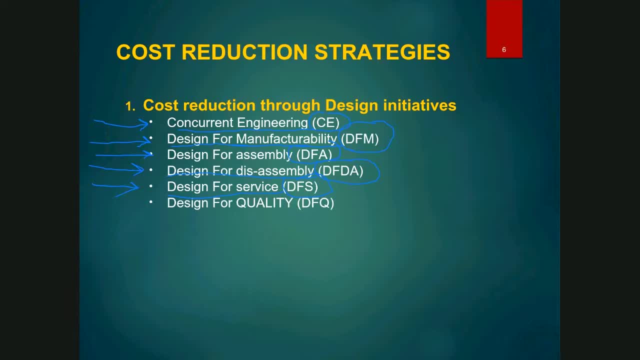 but what happened in my case- and this is a good example of design for service not being applied- is my. at one point i had the car for about a couple of years and the fuel gauge stopped working. i said, no problem, i can fix this, i'll just replace the fuel gauge. i started looking under the hood for the fuel gauge. i can't find it. i looked in the service manual for my vehicle and i find out that the fuel gauge is built inside the gas tank. how the heck am i my fuel gauge? i can't, i had to bring it in. 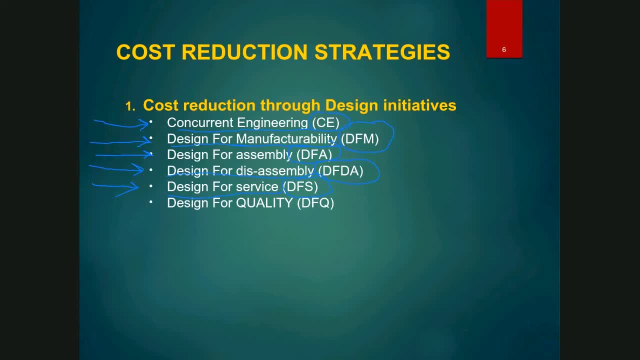 to the dealer. the dealer said: oh well, this is uh a long process because i have to, we have to take, put your car up in the hoist. obviously we have to disassemble your entire gas tank. we have to open up your gas tank and they're sealed, so we it's not easy to open them up and only then can we replace. 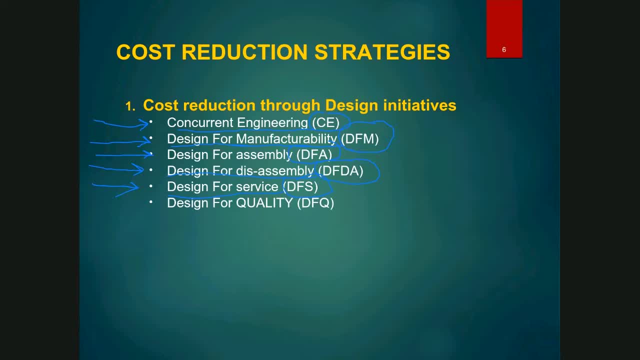 your fuel gauge. and i said that's going to cost you thousands of dollars. and i said, pardon my french, the hell with it, leave it alone. but i'd never bought one of those vehicles again in my life. i was so frustrated with that whole idea. so that's an example of not thinking about making 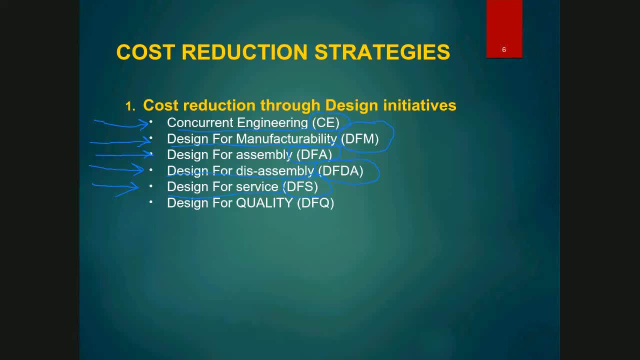 your products serviceable. and lastly, we also have to design our product in such a way that we can easily build it with good quality, so it's going to be reliable. so we'll talk about this one later on. so these are some initiatives- cost reduction initiatives- that we have to think about up front for our product. 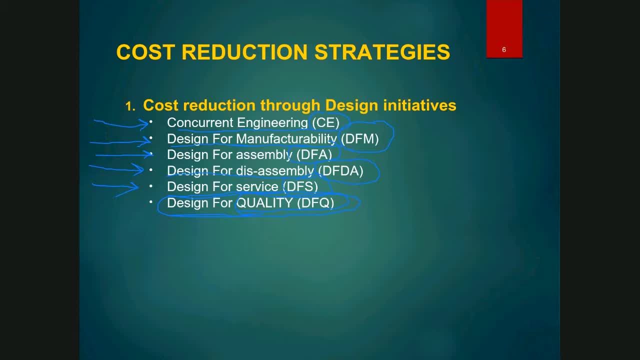 we have. our design has to be such that The product can be manufactured, The product can be disassembled. The product can be assembled easily, can be serviced easily, has good quality built in, Because if we don't do this, it's going to cost a lot to repair our products, to build our products, to make our parts. 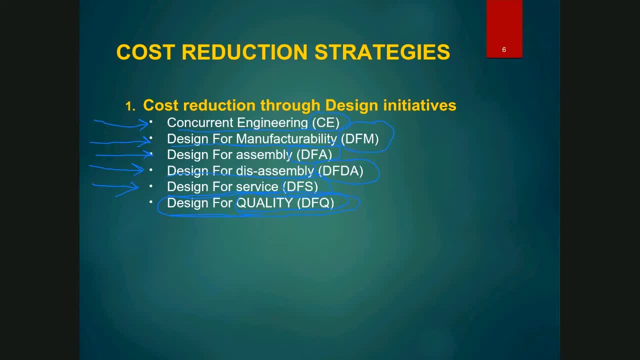 So at one time, as I said, I was in the design activity of Ford Motor Company, So I know exactly what went on with this activity and how important it was in determining what the overall costs associated with a vehicle were, What the vehicle line was at the end of the year. 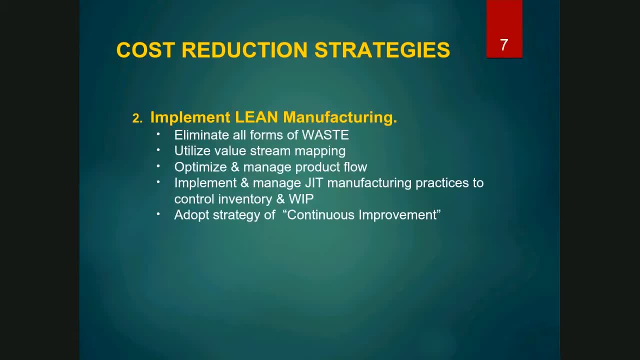 All right, let's move on to our next slide. Next, cost reduction strategy is something that we're going to learn about a lot, And this is called lean manufacturing. Now, this may not really be something that you know about right now. 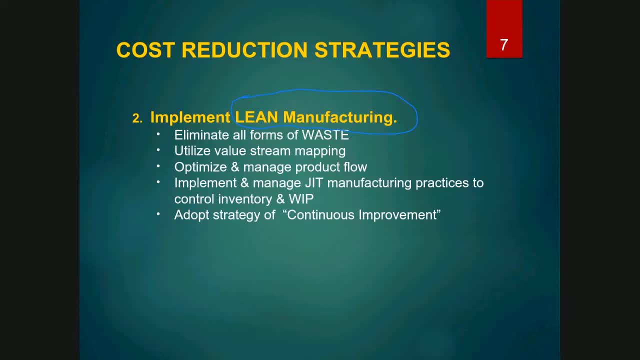 But rest assured, We're going to learn about lean manufacturing in the second part of our course. in the second- Yeah, the second half, I should say. But what lean manufacturing is all about is the idea of coming up with strategies and methodologies which will eliminate what are known as all forms of waste. 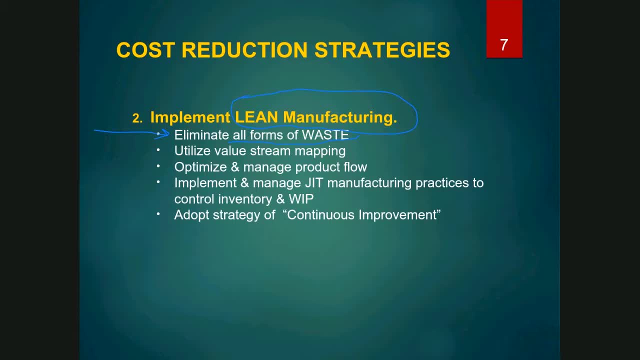 And you're going to see there's many forms of waste when we get there, And then we're going to figure out how we can eliminate the waste. We can utilize something that we call Value stream mapping. The idea is here is to how do we make sure that what we're doing is adding value to the product? 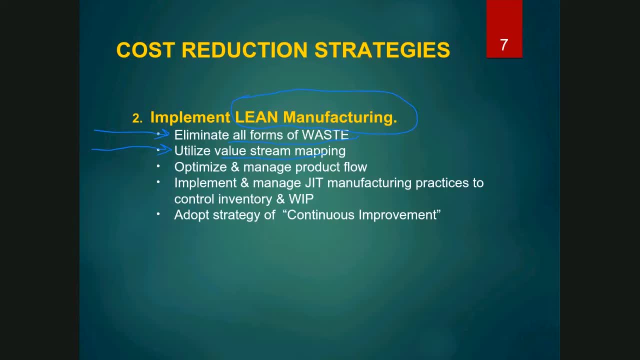 We're not doing something just for the sake of something, but we're actually adding volume value and we're going to do some exercises to see how we can make sure that we are always adding value, and what we want to do is eliminate the operations that do not add value. so 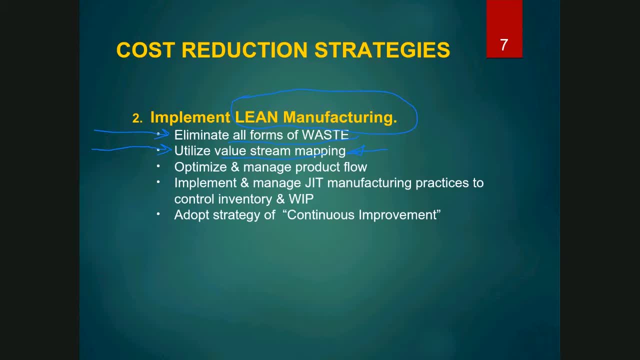 we'll have to understand what we mean by this. we'll see it later on in our course. next one: we want to make sure, by practicing lean, that we optimize and manage product flow. so this we're going to learn very, very soon when we learn how to plan for let's. I'm going to call it layouts- floor plan layouts- so we're 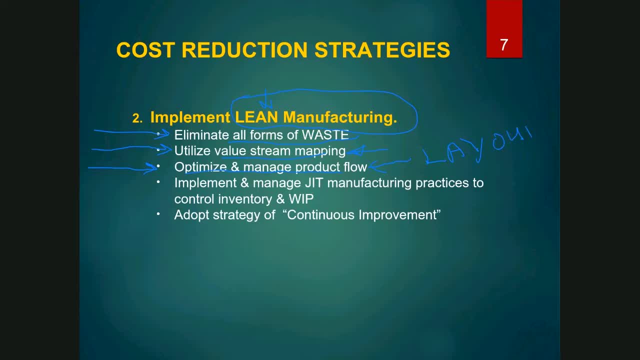 going to be discussing this very shortly, maybe in the next week or two, and we're going to talk about how we create effective layouts. the next consideration of lean is to use what is referred to JIT. what JIT is is an acronym for just-in-time manufacturing. we'll see this is a very important 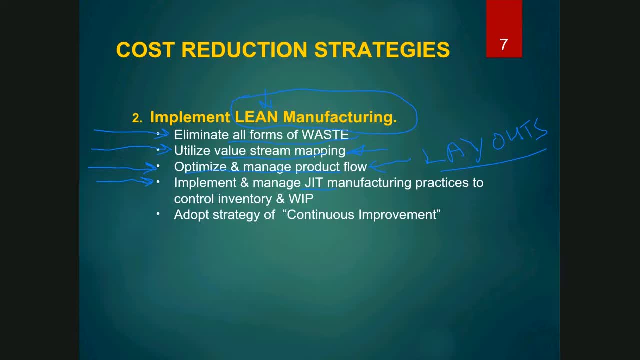 component, making manufacturing operations very efficient, and also how to control inventory in the plant, because we're going to see that inventory costs a lot of money so we want to minimize it. and this acronym here WIP, W I P- this stands for work in process, so typically in a manufacturing operation or in a, we have 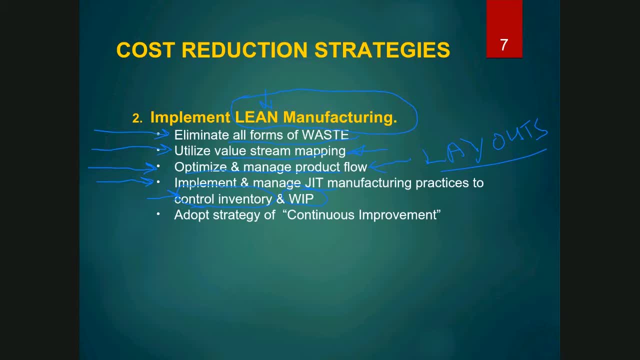 three stages. so we have a talk here where we have the raw materials. we have the raw materials. that's the raw materials per unit, right? so what we have here is the products that we have the raw materials. I call it. we have the raw materials. that's all the stuff that we need to make our parts. then we have the finished. 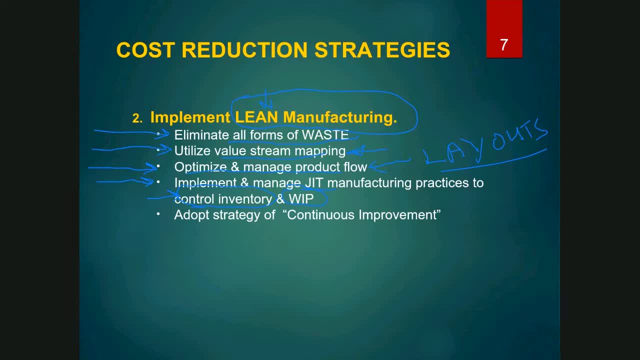 product, which is what we're going to give to our customers, and everything in between we're to as work in process. so JIT, just-in-time manufacturing- helps us to control both our inventory and our floor in order to be able to use various products, and that means we're going to have to set up a lot of dois. we're going to 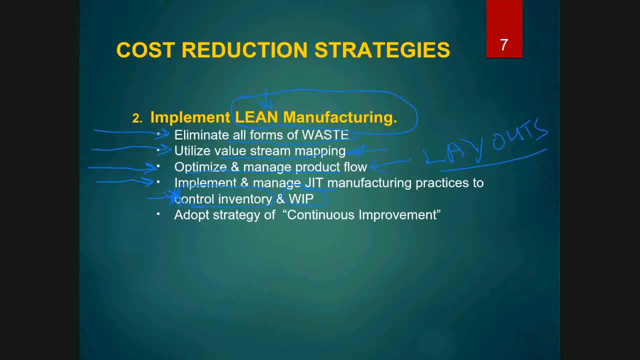 inventory, raw materials and also finished goods. not only that, but also whatever is in process. so a very powerful strategy. and, lastly, we also always have to have a strategy for continuous improvement. so many companies put together what they call- and i'm going to use a term here- that's. 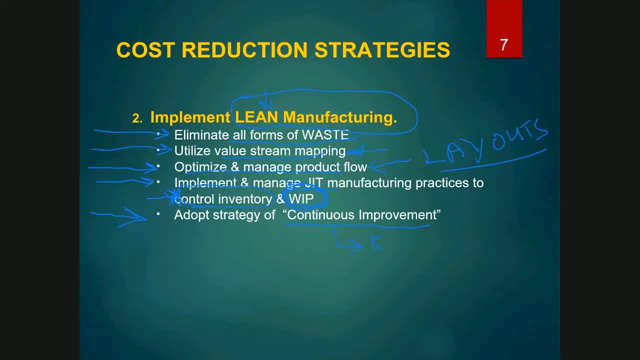 probably very foreign to you. this term is called kaizen, so kaizen is a product of, is a term is a japanese name which they use for cost reduction teams. so they put together a team and they go looking around and try to identify cost reduction opportunities. so we'll talk about that again later in the course as well. so this is our 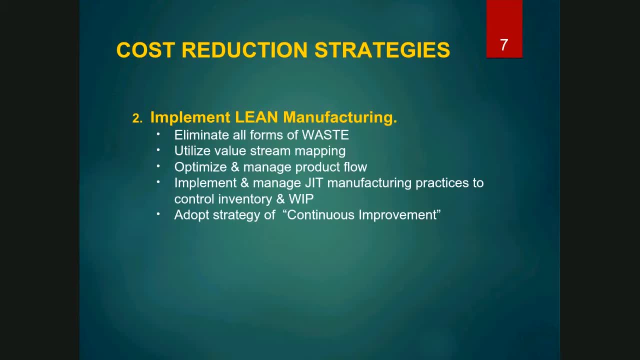 second approach to reducing cost, that is, the implementation of lean manufacturing, which involves, by the way, all of these things and more. these are not all inclusive. when we do the unit on lean, we'll see there's more to lean than just this, but these are the primary things. 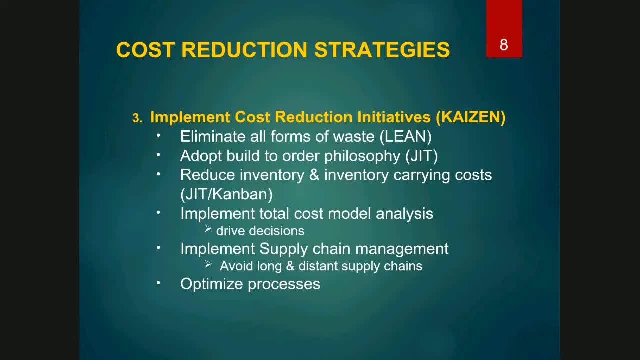 all right, and here's the term kaizen, so that i used earlier, so here we have. the third strategy is to implement cost reduction initiatives by using the term or the approach of kaizen, which, as i said, really they are cost reduction initiatives driven by teams that are set up to look for cost reduction opportunities. and these kaizen teams, 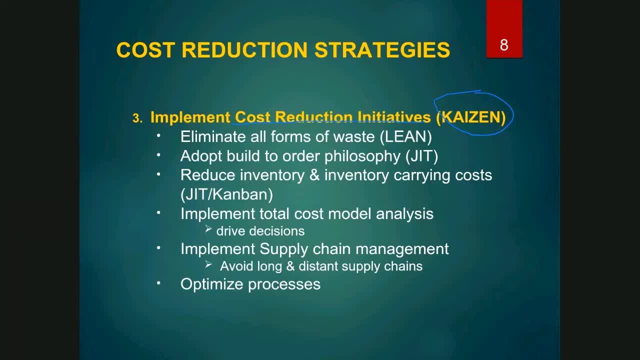 they work on trying to eliminate all forms of waste, which is part of lean. they try to implement what is called the build to order philosophy, or just in time. uh, try to reduce inventory by adopting not only just in time, but a tool, a specific tool, which is called a combat. again, we're going to see czar, so don't get excited. 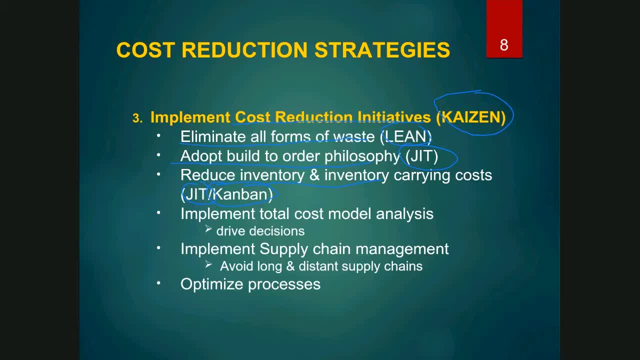 or anxious. if you don't know these terms right now, we're going to be talking about them. uh, we want to make sure that we implement what is called the total cost model to drive all our business decisions, and we're going to talk about the total cost model as well. 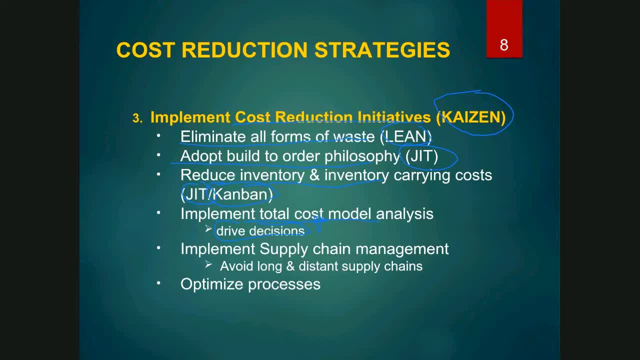 so not again, don't stress right now: uh, we're going to visit a reduction, cost reduction strategy that we refer to as supply chain management. we want to make sure that our supply, we avoid long distance supply chains because they're costly, and we want to learn how to optimize our processes. 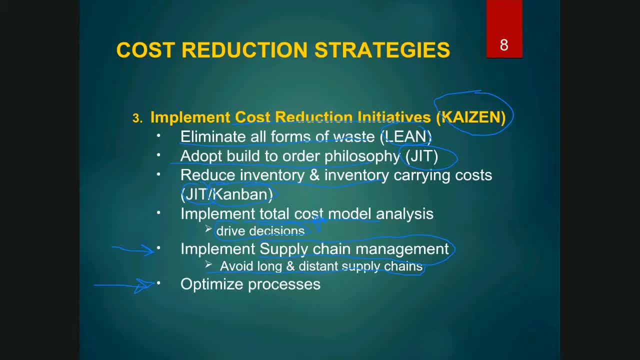 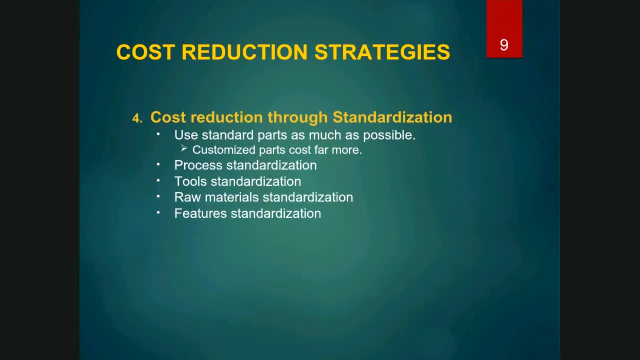 all to follow all right cost reduction. Cost reduction through standardization. so we kind of talked about this at the very beginning, where we said the idea of moving from custom parts to using common parts. This concept was reduced by Eli Whitney back in the 1700s. 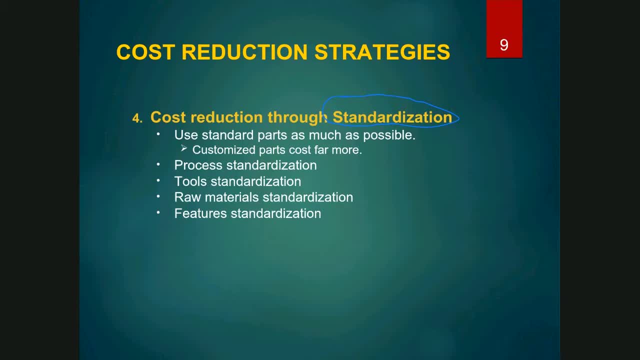 We still use that concept today. as I said earlier, at Ford we make a strong, or we made strong use of this idea. So when we designed parts for Ford cars, we try to make them common for all the Ford models as much as possible. 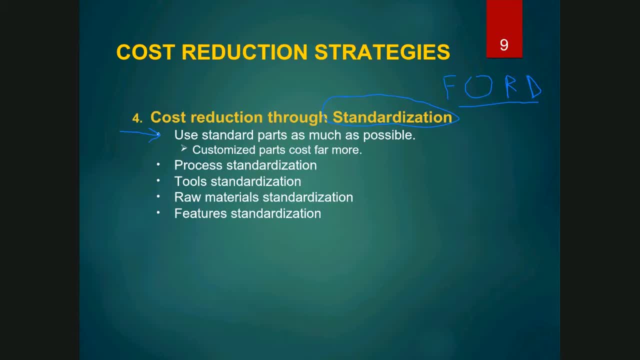 So here we have that very same idea: Use standard parts as much as possible, Because customized parts cost far more. Not only do we want to standardize our parts, we also want to standardize our processes. So again, when I was at Ford at one time, as part of my responsibilities, I was responsible. 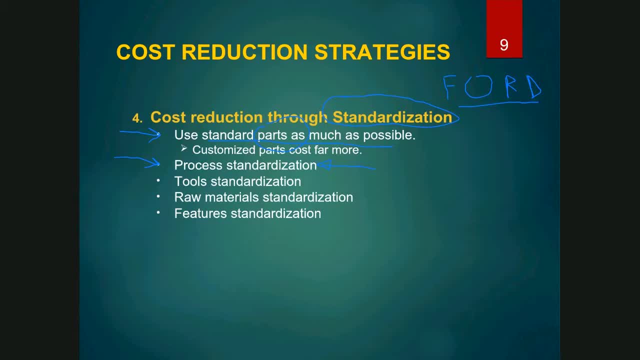 for the team- A part of the team that we went around from plant to plant to plant in many countries around the world that were part of Ford Motor Company and we would identify what are called- I'm just going to put it here- BIC. 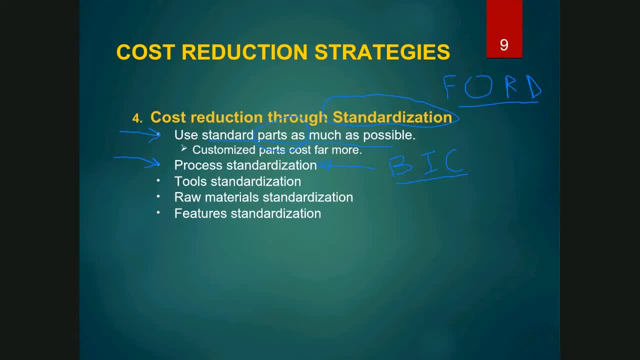 And what that stands for is best in class. Okay, Processes right here. So we would go, let's say, to plant A, and we say, oh, we're ready. This process that you're doing is the best we see everywhere. 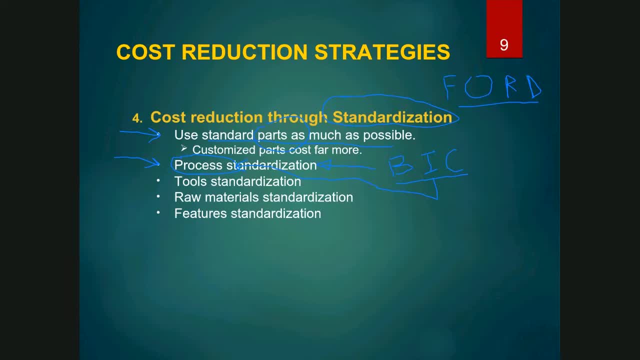 So what we're going to do is take this process and call it: this is the best in class, And then what we're going to do is take this process and make sure that everybody, every other plant, does the same process. Okay, We do the same thing here. 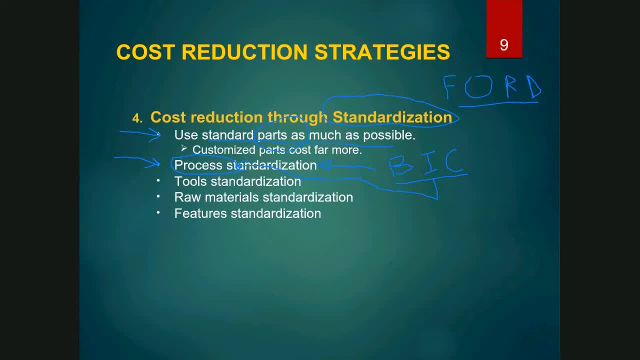 We take part. we do the same thing here. What we're going to do is we're going to figure out better ways to make these parts. So we adopted best-in-class strategies or best-in-class practices. First, we were work with a team to develop them, and then we would implement them everywhere. 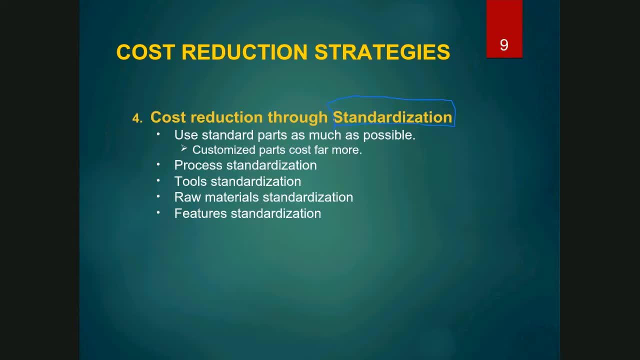 So again, the idea here is we want to standardize as much as possible everything we can: processes, tools, raw materials and the features or options that we put in our products. So all of our models should have a set of standard features. 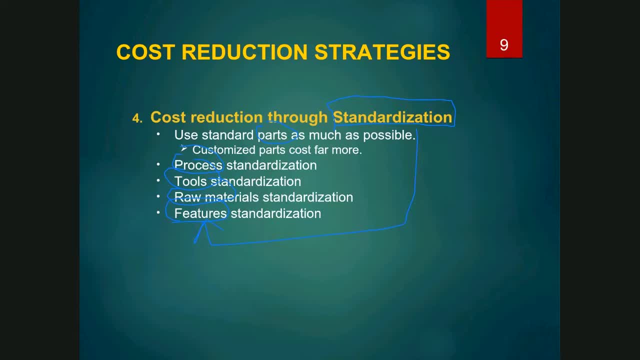 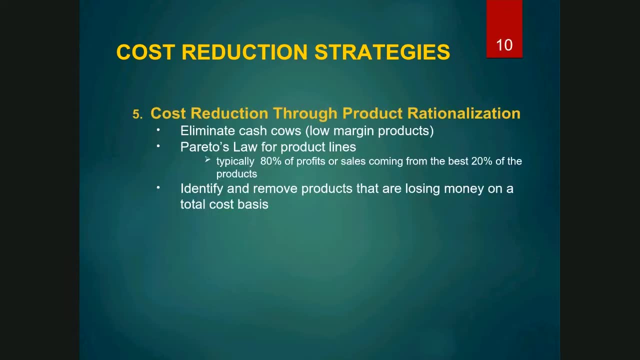 Then if you go to a higher model, you have more features and so forth, And that next cost reduction strategy is one that we call product rationalization. So I remember in one of the poll questions I said: making as many products as possible. 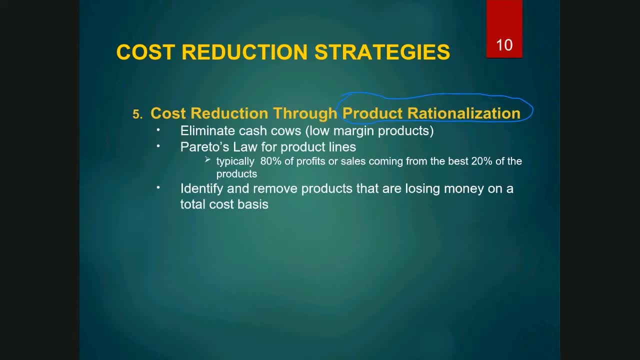 Well, that was kind of a tricky answer that I gave. I'm going to give you a reply there, because right here I'm suggesting that we should eliminate products that are cash cows, which means they have low margin products. So if we're working a company and we're making, let's say, a hundred products and 50 of those, 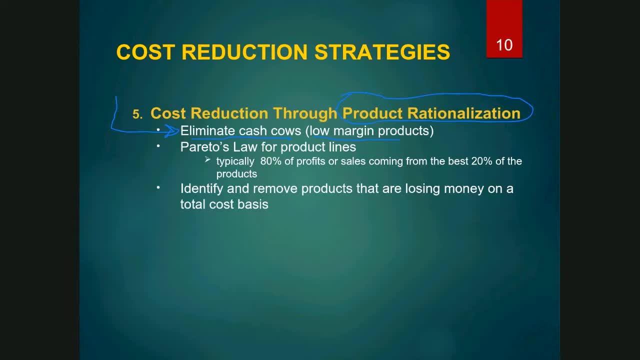 products we're barely making a profit on, or we may be even losing money on it. then why are we making those products? Well, we should make our products where we're making profit, where we're making money. So an interesting concept. this gentleman here, Pareto. he was an Italian economist. 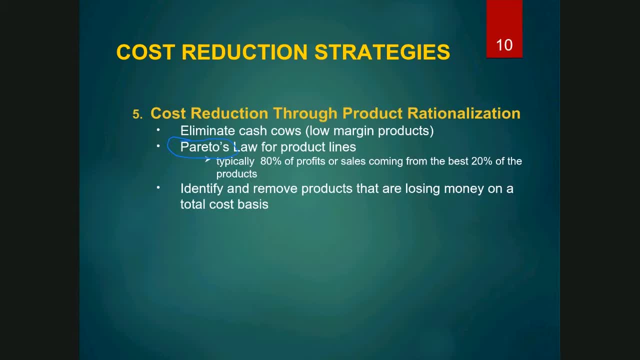 He came up with this law for product lines And he said that in most cases We find that 80% of profits come from only 20% of our products. So that means we theoretically can get rid of 80% of our products and only make 20% of. 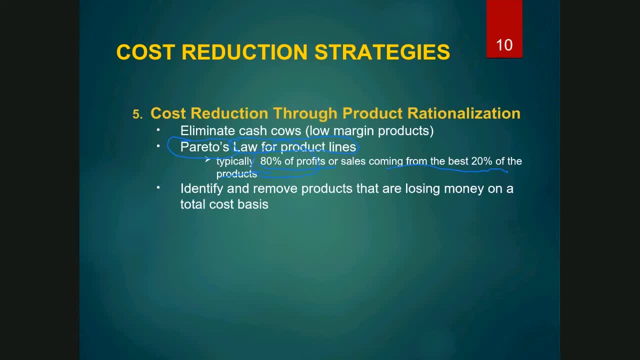 our products and we make 80% of our profits. Okay, So this is a very powerful idea And that's why we should think about this step number one, And if we think of this approach, then we should identify and remove products that are: 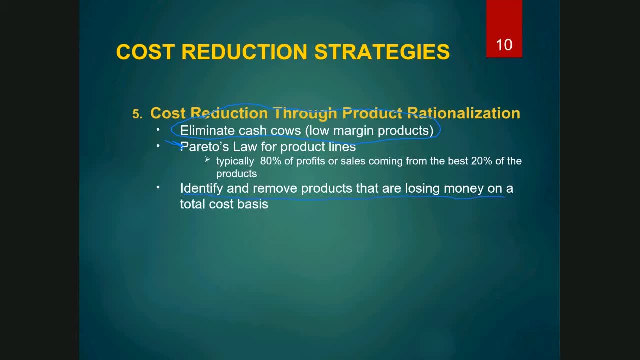 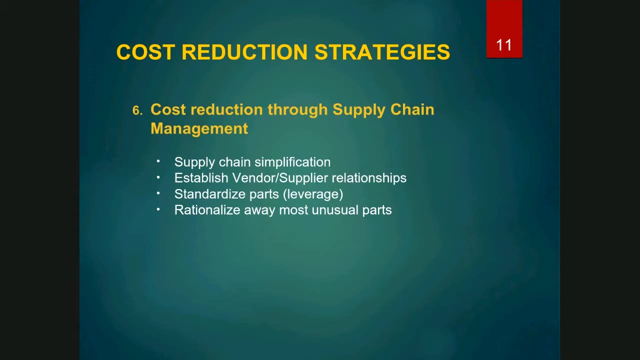 losing money on a total cost basis. So we'll talk about total cost later. Bye Bye. 1. By using one of the things we talked about earlier, which is the value stream map, We want to make sure that we have good vendor supplier relationships. 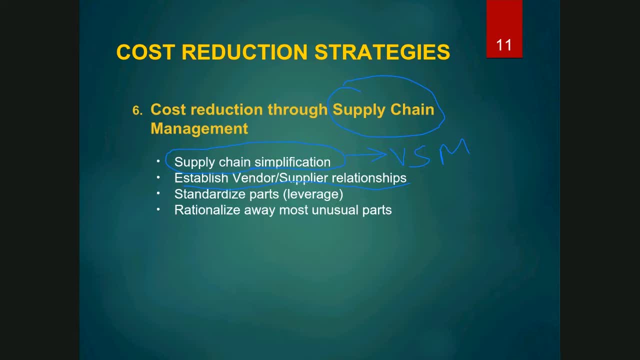 We want to make sure that our suppliers use the same cost reduction strategies that we use. We want to make sure that our suppliers use good quality 1. so when we get their parts, we're going to have good quality. we want to make sure that the 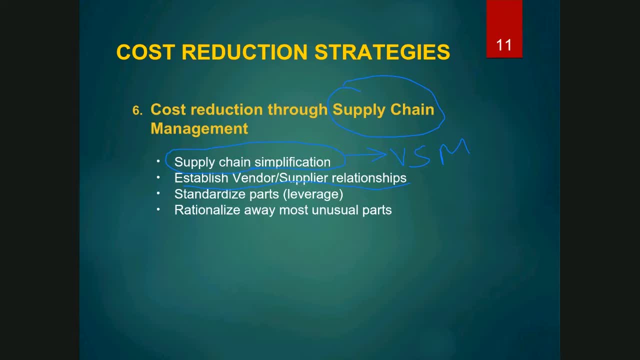 suppliers apply lean strategies. that way they're reducing their costs and we can have cheaper products to put in our products. we want to make sure that they use standard parts, common parts, so then we can buy many of the same parts that we can use across our product lines, and the more we 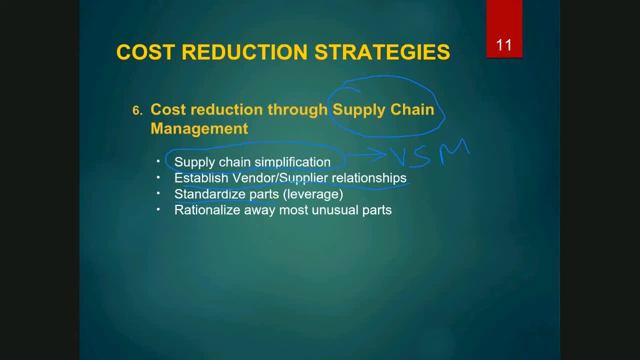 buy, the more leverage we have and the better price they can give us. and along with idea, we want to get rid of all the unusual parts, because suppliers usually caught charges a lot of money for strange parts or parts that we only will need a few of, and they have to make them. that cost them is a lot of. 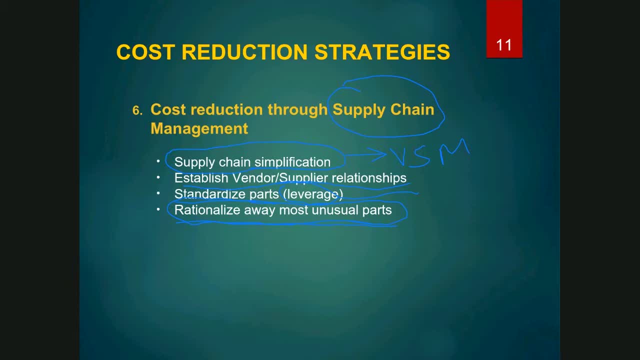 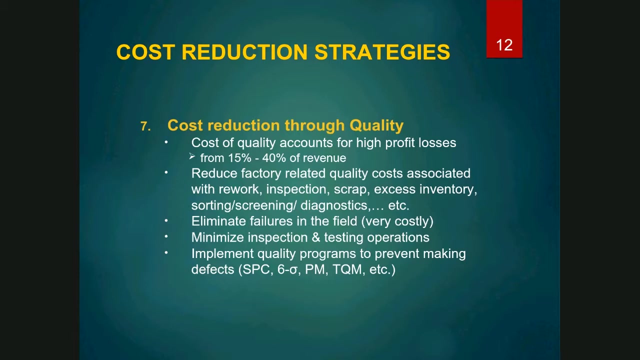 costs them a lot of money. okay, and one more- this is an important one- we can reduce. we can reduce a lot of cost by making sure we build good quality. I want to put an asterisk on this one, because I think it's important that we have a good quality product, and we want to make sure that we have a 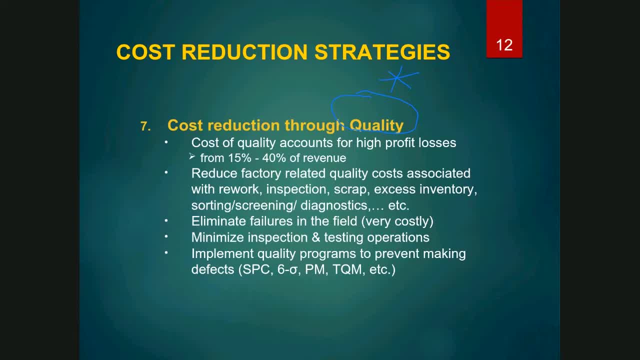 good quality product and we want to make sure that we have a good quality product and we want to think it's one that is often forgotten, or at least the opportunity that exists. within good quality, building good quality, there's a lot of opportunity to reduce cost if we do it correctly. 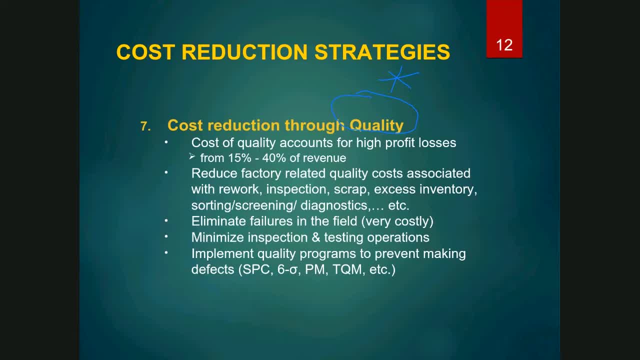 it is noteworthy that in point number one here, the cost of quality can account for high profit losses in the range of fifteen to forty percent of revenue. that's very significant. what this means is if we build bad quality, we can spend about that much or lose about that much because we did that. 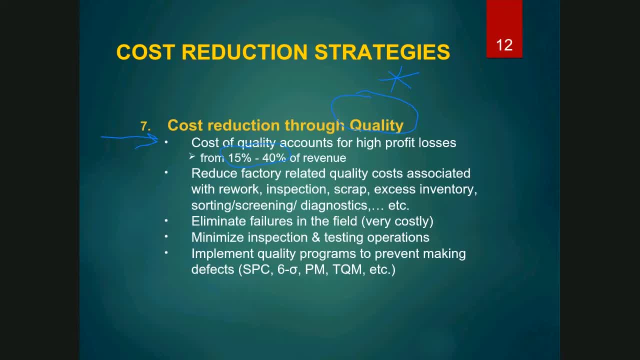 so, if that's the case, we have to be very diligent about you, reducing factory related quality costs that are associated with rework, inspection, scrap, excess inventory, sorting of bad parts, screening of our products, diagnosing our problems and so on. why do we have scrap? why do we have to rework? 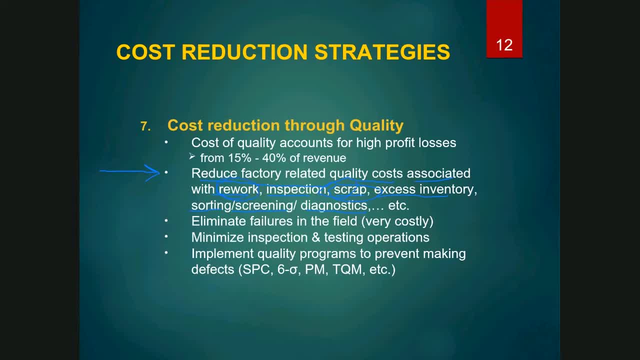 why do we have to inspect? the answer is because we're probably doing doing it right. our processes are not good enough, so we generate scrap, or we have to fix our problems by rework, or we have to troubleshoot through diagnostics to try to figure out why the product is not doing what we wanted to do. 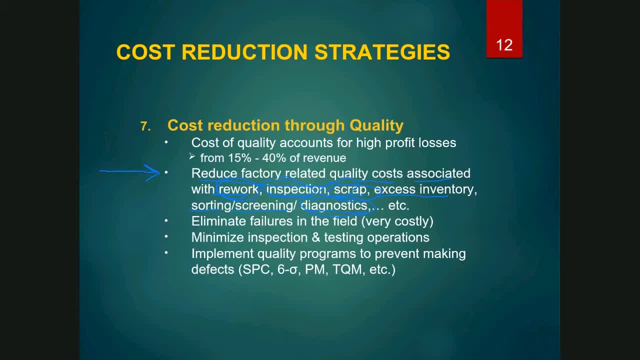 so these are all very costly. so we have to make sure that our quality is good right from the beginning. that way, we can eliminate costs associated with quality or bad quality. here's a good one. we have to eliminate failures in the field. this is extremely costly. what do we mean by failure in the field? so think of it this way: while we are building our product, 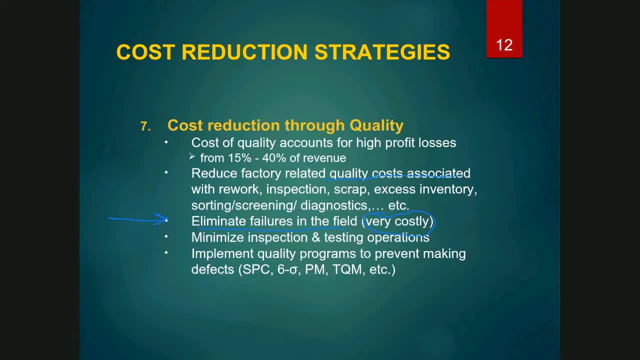 in our factory. that's still in our control. so if we find that when we do our troubleshooting or our diagnostics on the product and it's still in the factory, well we still have it there, so we can fix it there. it may it's going to cost us to fix it, but it won't be nearly as bad if our product 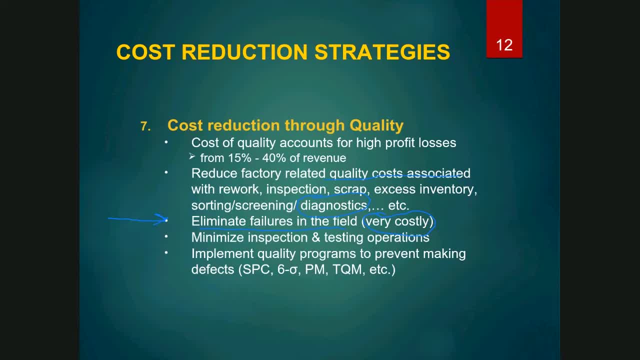 goes out to the customer and then we have to fix it. so again going back to my time at ford motor company, it gives us a very good example for this. so let's say we were in the process of assembling the ford mustang in the ford body and assembly plant and we find, while we're assembling, 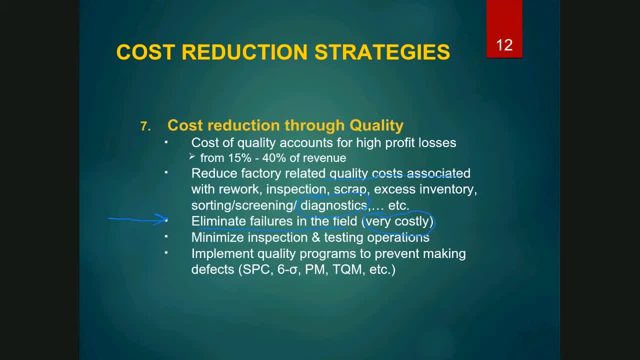 it that there's one part that's not aligned properly so clearly. once we find that we have to fix that part, the big car parts are right there. the chassis of the car is coming right down the line, so all we have to do is take it off and replace the part that was faulty. 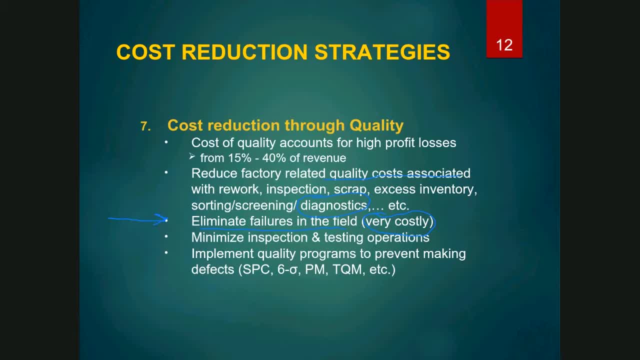 so in itself that is costly and we should try to avoid that by doing it right to begin with. but what would happen if we don't find that problem while we're building the car? and we complete the car, we think everything is okay, we send it to our dealer. 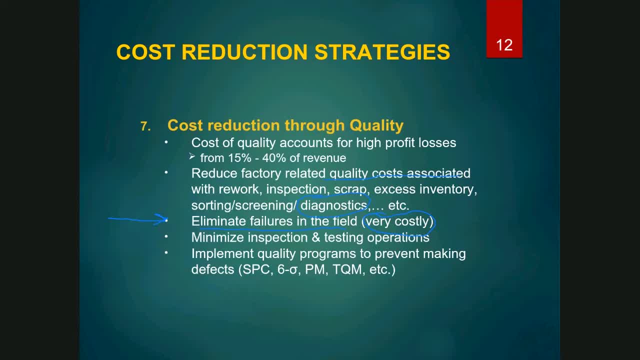 then our dealer sells it to a customer. the customer takes it home and, as they're driving down the highway, the car breaks down on. well, guess what? at this point? number one: we have a very, very angry customer. they may never want to buy our products again. number two: we have to go out and fix that car. 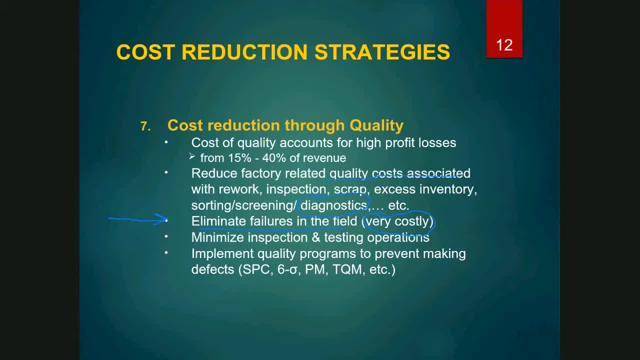 which means we have to go out and get the car. we have to bring it back to our dealer. the dealer will try to fix it if he can fix it. if he can't fix it, he has to bring it back to the fourth plant and the fourth plant has to fix it. then from the fourth plant it has to go back to. 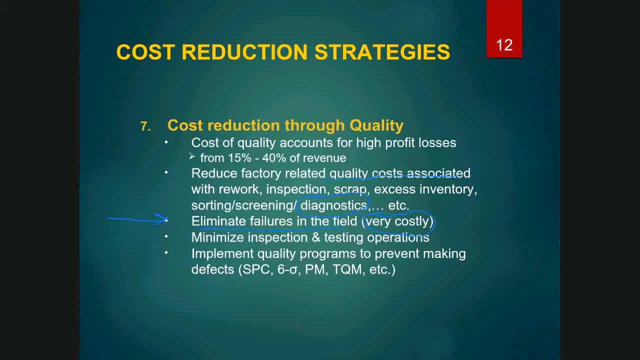 the dealer, from the dealer has to go back to the customer, which may take a long time, and throughout all this time we have to give the customer another car, so he has a car that's going to go back to the dealer, so he has a car to drive. he or she has a car to drive. 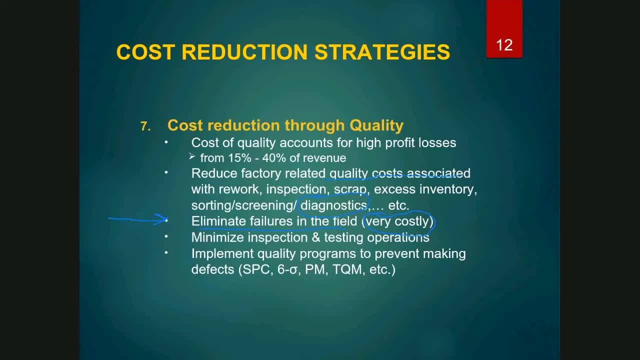 so can you imagine how much that would cost ford motor company if that were the case- very, very high cost. we used to tracks with incredible aggressiveness because whenever there was a field fader wait, somebody's head was on the line. we can't have to field failures. it was that important to us at ford, and that's true of anybody, so this one is. 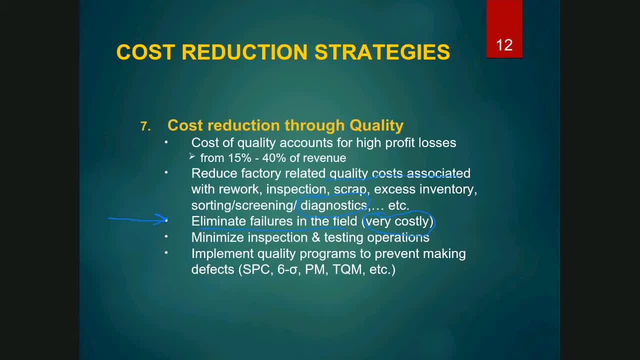 a very important one. all right, i think i beat that one enough. uh, next one: we have to mint over here. we have to minimize the inspection and testing operations that we do in our in our factory. why do we have to have so much inspection? why do we have to have so much testing? 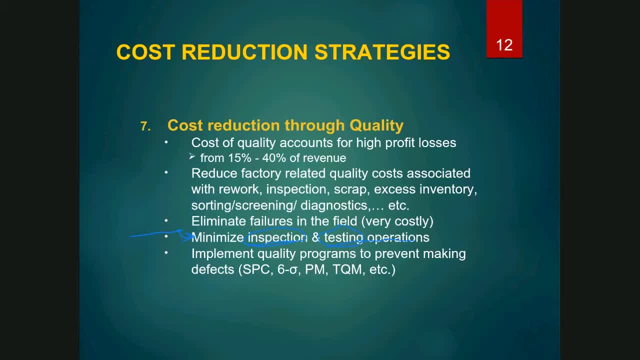 these are called non-value-added operations. we have to do it because obviously, the way we're doing things is not very, it's not perfect, it's not optimal. so to make sure that everything is working right, we have to inspect and we have to test. we should get rid of all of this by doing. 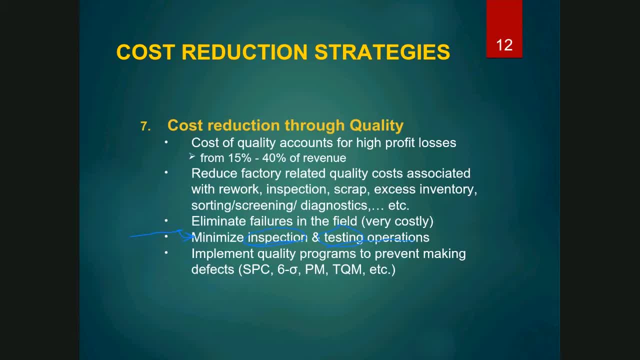 it right from the beginning. we're going to talk about a lot more about this later on. and lastly, over here we want to make sure that we implement the inspection and testing operations. we have to Implement quality programs to prevent all of this stuff that we talked about up here by doing statistical process control, quality programs, Six Sigma quality programs, preventative maintenance programs, total quality management programs, et cetera. 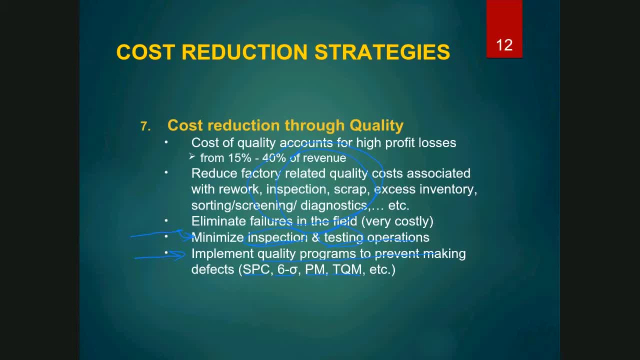 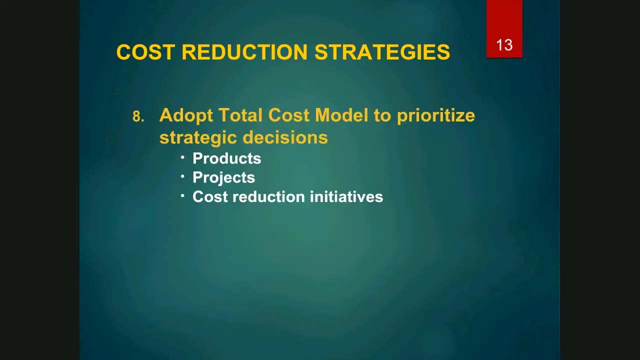 So I'm very big on quality, Very big. It has to be done right from the beginning. All right, And the last thing I want to talk about cost reduction strategy is whenever we have to make a decision- a decision about products, about what projects we're going to work on, about what cost reduction initiatives we want to produce- 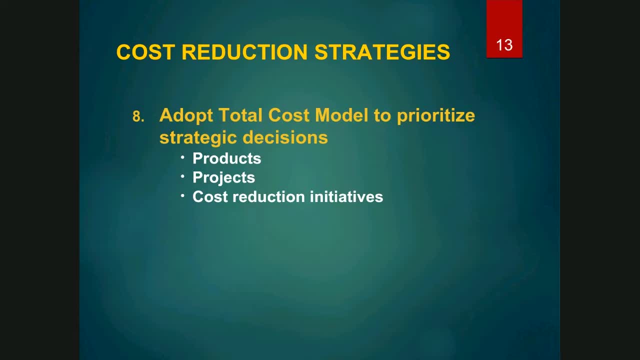 we want to make a decision. We want to make a decision We want to prioritize or work on. We have to use something called the total cost model, And this is quite an easy model. in concept. What it means is, when you look at your products, look at what the total cost model tells you. 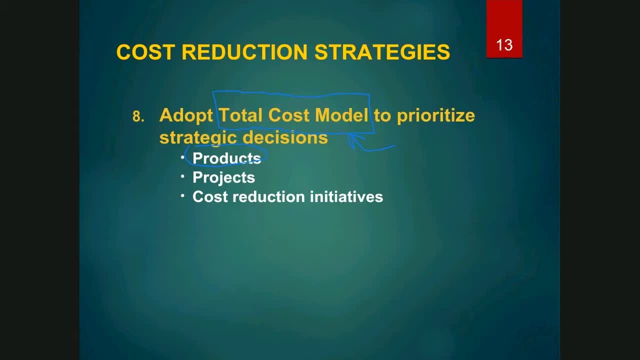 The products that contribute most to your total cost are the ones you want to keep, The products that you want to keep. the products that lower the total cost you should get rid of. The same idea applies to products. If products increase our total cost model, that means we're improving. then we prioritize those products. 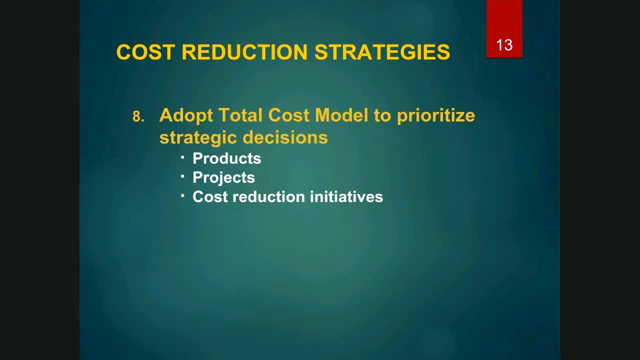 Okay. And lastly, the same idea is: if we have a project or let's say we have a team of engineers and technicians working on cost reductions and let's say they have 10 good ideas to reduce costs, but we don't have enough people to work on 10 ideas all at once, where do we begin? 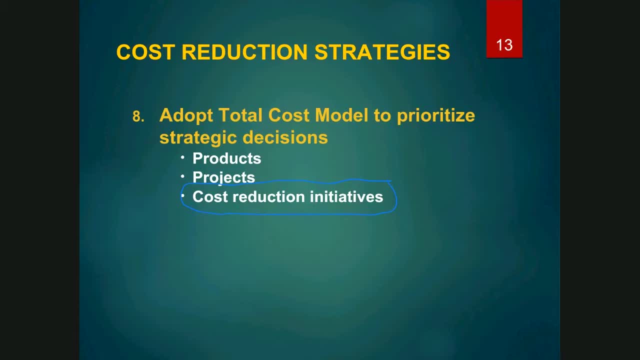 Well, let's start with the idea that affects this one the most. So, if we can reduce our total cost, the idea that reduces it the most is the one we're going to begin with, and then we were going to prioritize them accordingly. 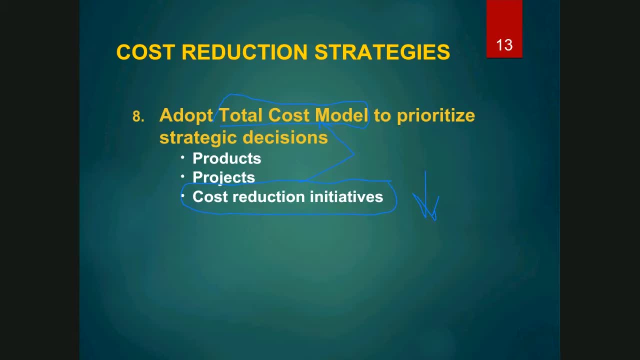 So maybe we can only work on the top three, top three, T3.. And once we take care of these, Then we'll look at the next three. They become the top three And once we can fix, can do these, we'll tackle another three. 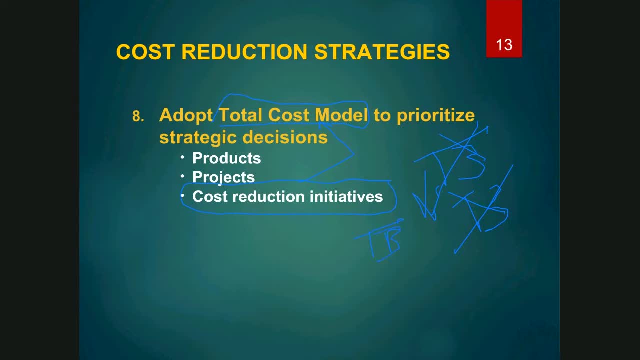 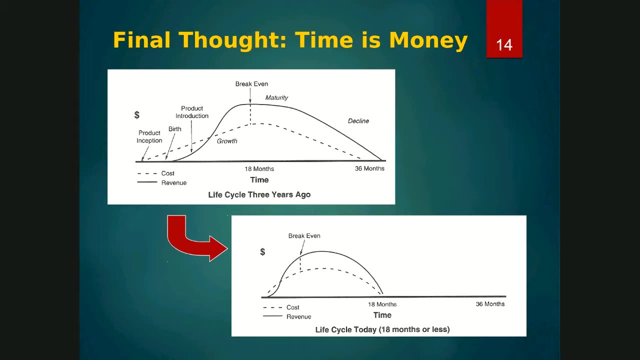 Oops, you get the idea. Okay, I have one more slide here for you that I want to talk about today, and then we'll call it a day, And this slide is an interesting slide. So, remember, one of the things we talked about in one of the earlier slides was the idea of introducing product from the time we think of an idea to the time we get it to the customer. 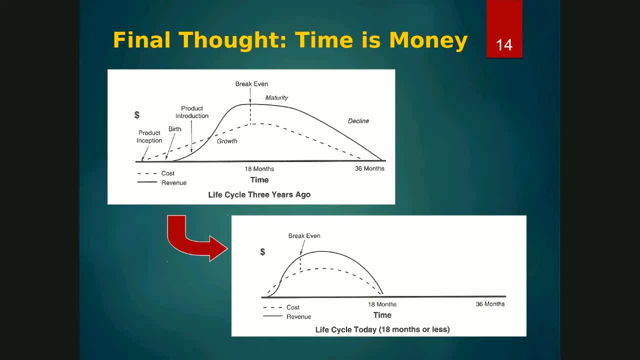 And we call that CTC Concept to customer. So the idea that we're looking at here in this slides, and I have two graphs here That I want to talk to you about briefly. Let's focus on the top one. So this graph represents the life cycle of a product. 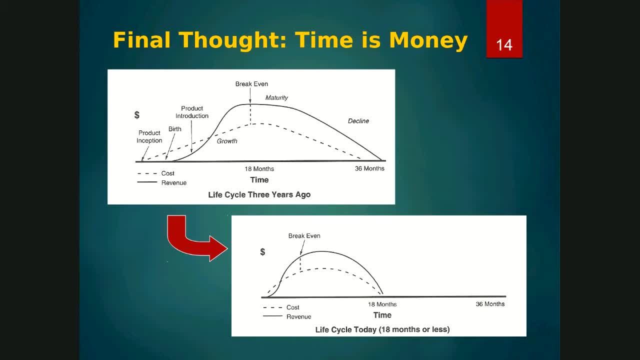 You see that on the graph there's two curves. So we have the solid curve right here- This is the revenue curve- And then we have This curve, The dotted line, which is our cost curve. So let's look at these for a moment. 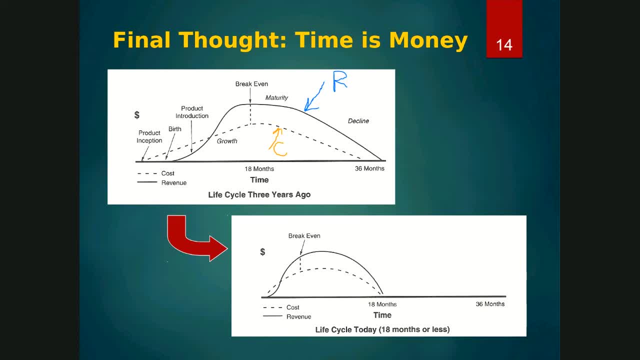 Let's see what happens, first of all with the cost curve, which is the dotted line curve. So I'm going to keep my orange color for that one. Okay, You see here that when we begin, here's our product conception, our product idea. let's say: 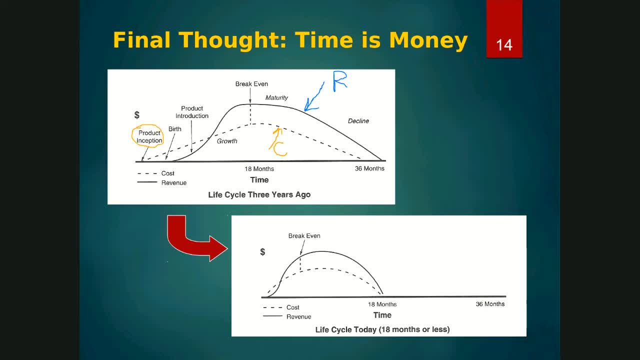 And then you know, we go through the product design, the development, all of this kind of stuff. We introduce the product, We build our first samples, for example, And as we go through this cycle you see that the costs are ramping up. 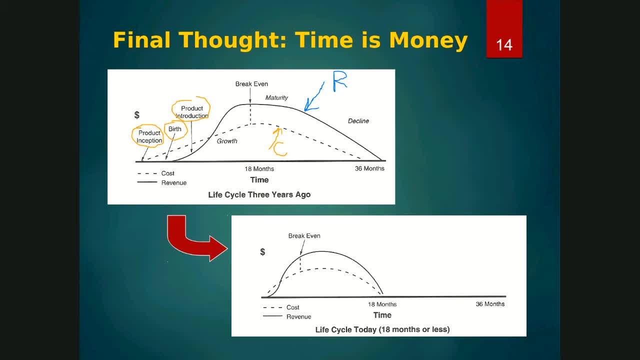 Okay, Ramping up, And then we do cost reduction initiatives And our costs start to increase And the curve looks something like this: Now you notice here that we have- let me just change my color for a moment- here. We have here a timeline. 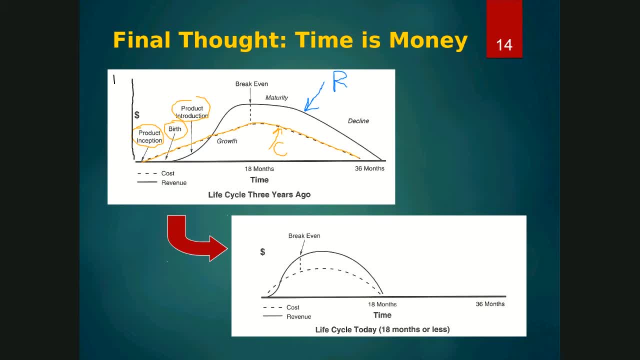 This is the start. I'm going to call it T0.. And here we have, let's say, the end of the cycle of this product, And I'm going to call this T36.. Okay, So T0 is time zero. 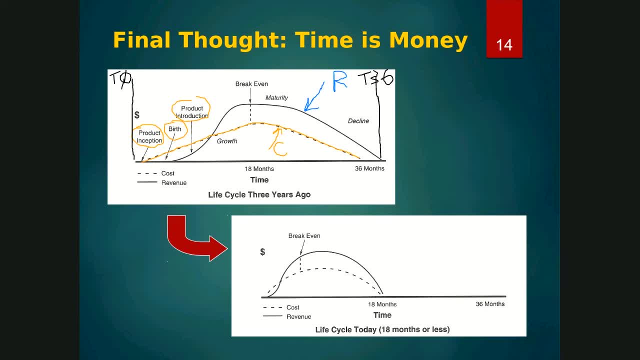 We begin everything We come up with, the idea. T36 is: this is months, So this is three years And the product And the product is phased out as this time. So we have these cost curves that we just saw. that looks like this: 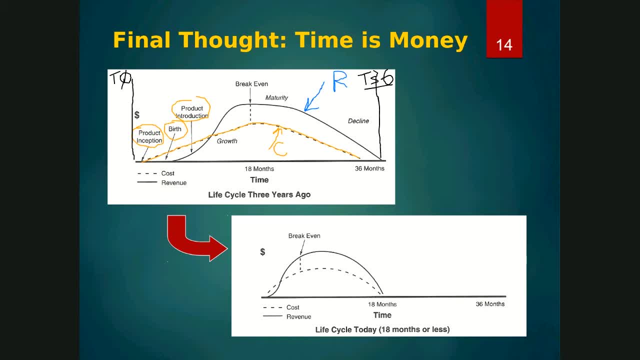 And let's now look at the revenue curve. You see that the revenue curve: at the beginning we have basically no revenue, So all we have is lots of costs here. We're incurring cost all here, all in this area. Then our revenue curve, which is the solid black line: as we increase our sales, we start ramping up with our revenue. 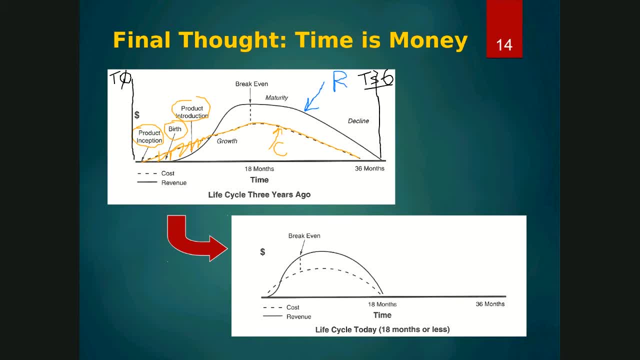 And we get to this point here, which is called the break-even point. That means that our revenue equals our cost, So R equals to C At some point. And then, after this break-even point, it means that we're making money. 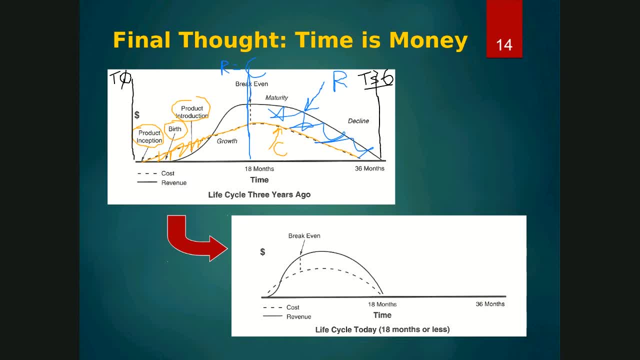 So, from a time of T0 to a time of T36, the difference between the revenue curve and the cost curve equals: what Profit? Now let me clear the list that I made. So in three years, let me just do this In three years. 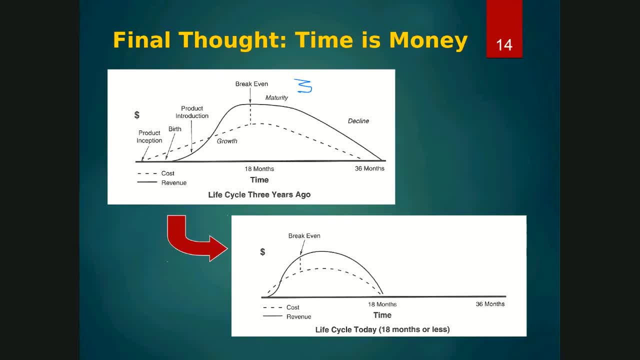 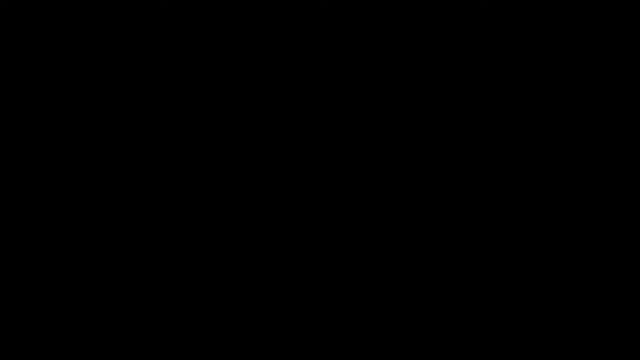 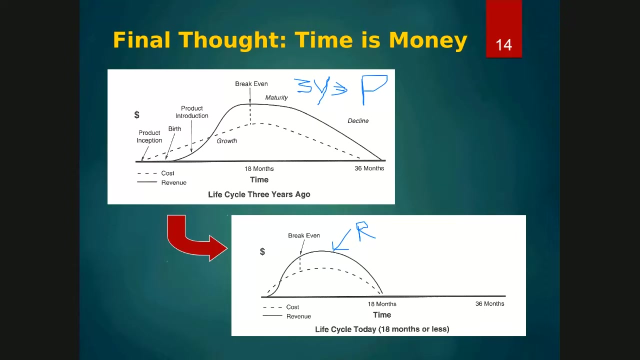 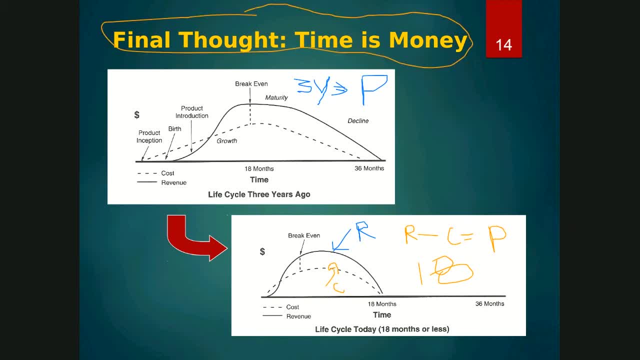 money and that's why I remember when I said at the beginning when I was at Ford, the lifecycle of the product initially was at four years, then they went to three, then they went to two Apple. they try to get an iPhone out there every year, sometimes even faster.